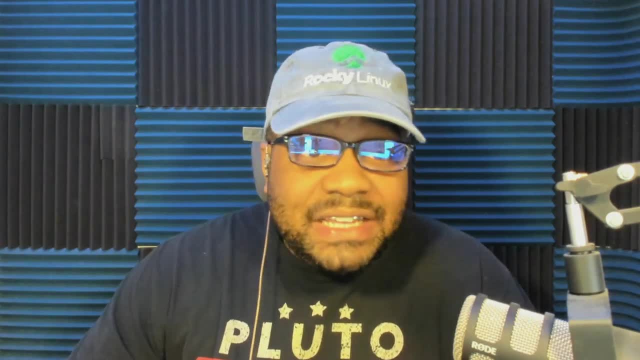 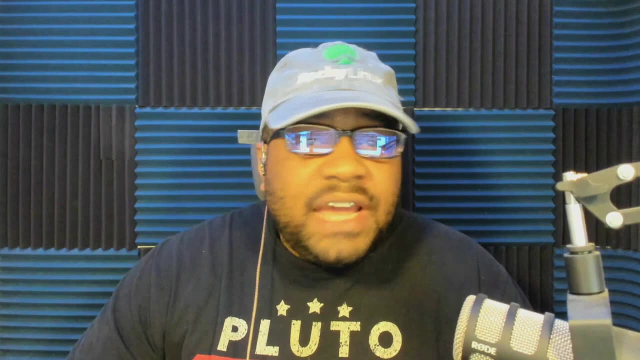 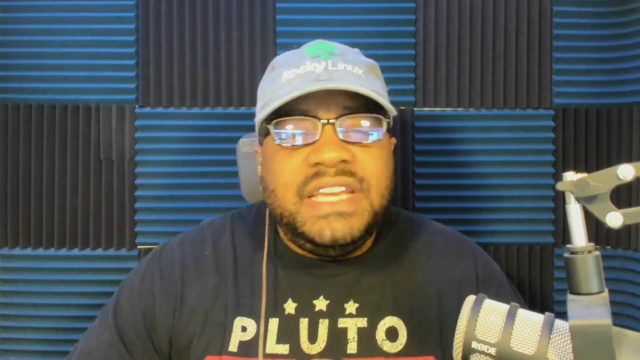 stands for so Tails, but it was designed to provide people with a level of anonymity and privacy when using the internet. and one reason how it does that is by the operating system made to run on a USB drive, and it doesn't save any files at all on the system. and one other cool feature about it: it 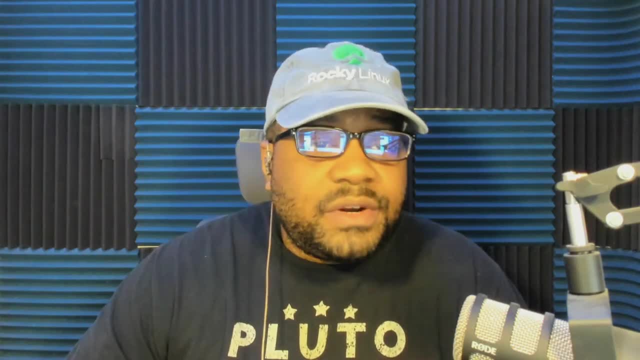 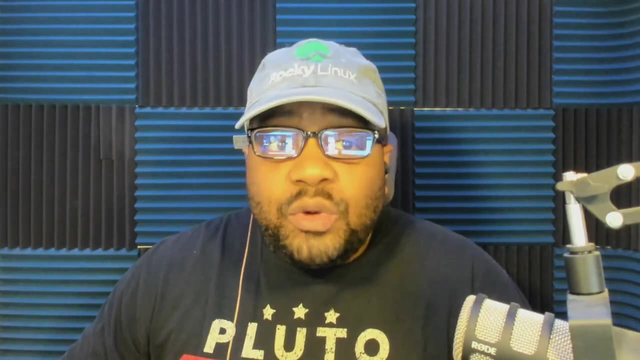 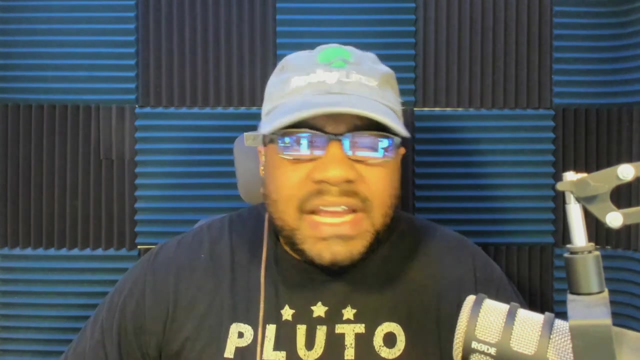 runs all its internet connections through the Tor network, and if you guys have never heard of Tor, Tor stands for the onion router, which is basically a free and open source software that enables anonymous communications over the internet. I can break it down a little more, but I do have a video on the Tor network and how it actually works. 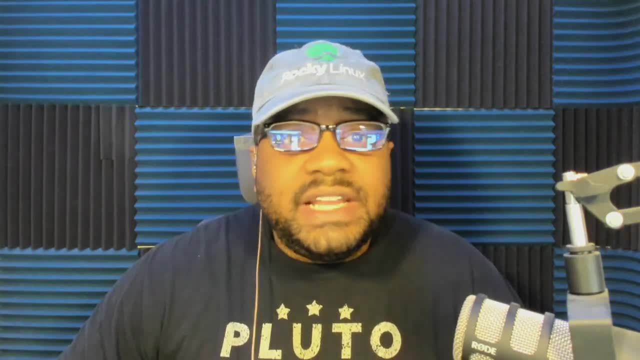 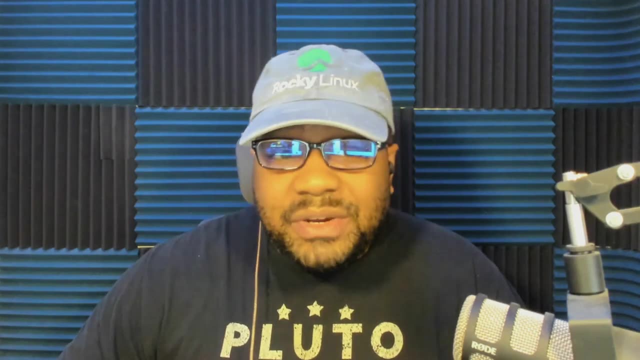 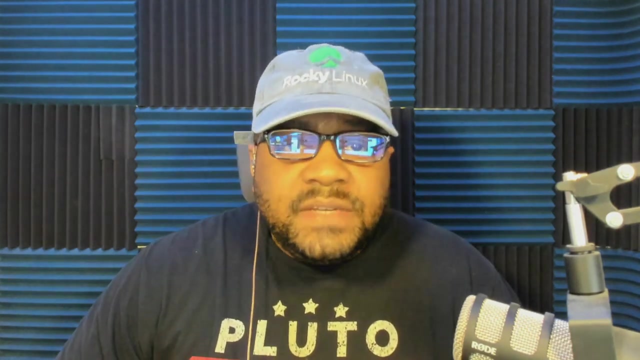 where I break down how the communication works on that network. but it's an awesome way of staying anonymous on the internet while browsing and doing everything else you want to do on the system. but some of the known security features of Tails is the encryption, the anonymity tools you know as 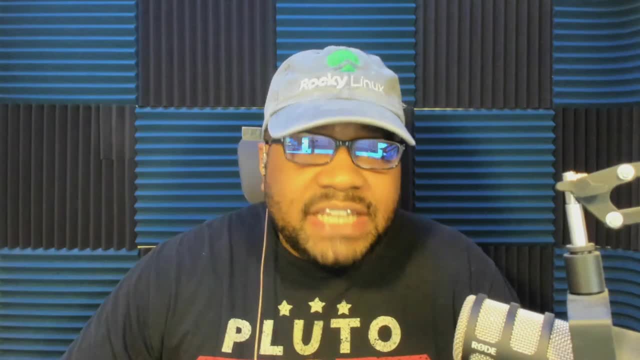 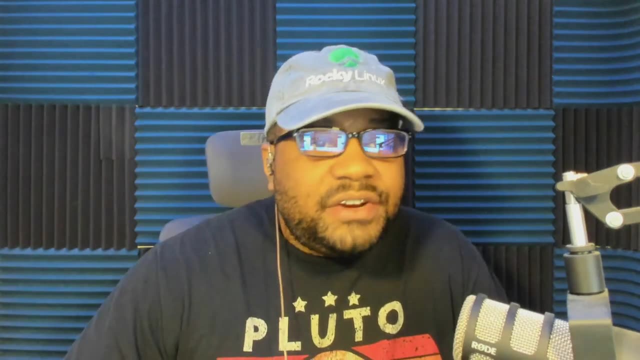 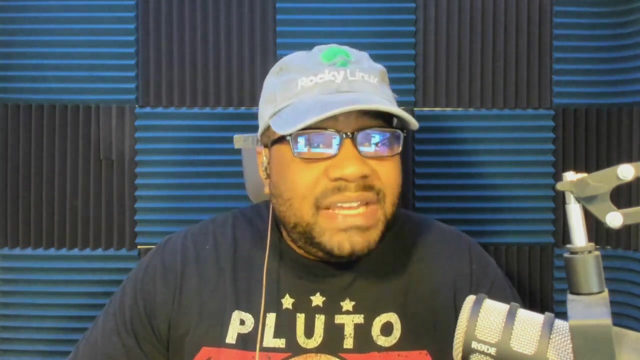 you know, like Tor, as well as secure communication tools like ricochet and a whole bunch of built-in privacy tools like https, everywhere, no script. you know thunderbird, with open pgp and the operating system. like I said it, it's made to run from a USB drive or you can also install it on a DVD drive. 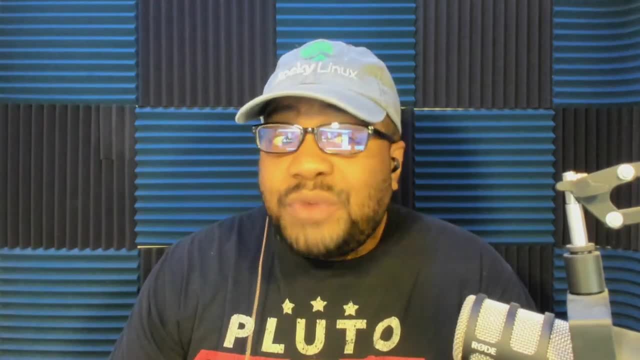 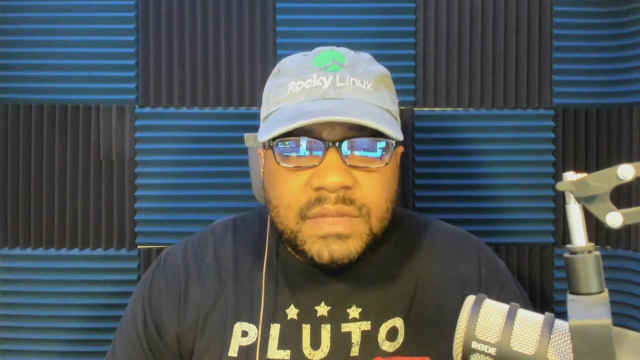 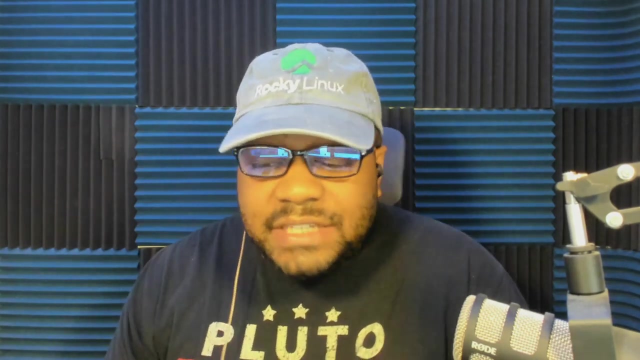 and I want to reiterate that all the internet traffic is routed through the Tor network by default, so that makes it super cool and anonymous. now, most of the people I hear that use Tor or like journalists or active activists, as well as people like you and me that want to protect their privacy. 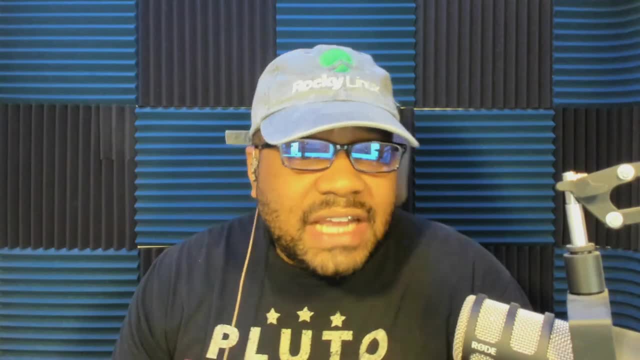 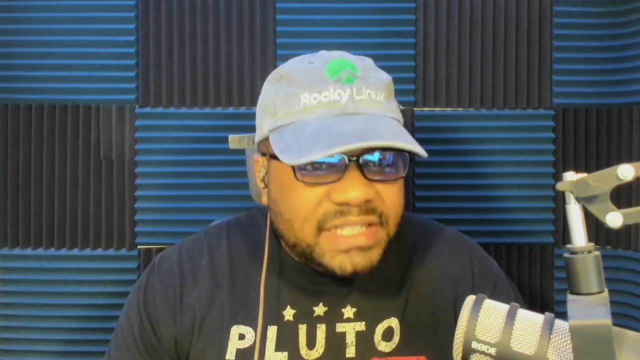 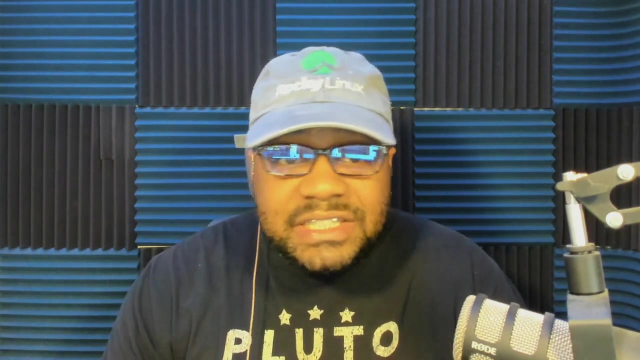 you may stay in a country that censors a lot of information. well, by using this operating system that kind of routes everything through Tor, you can circumvent that censorship by getting to sites that you typically wouldn't be able to if you weren't using this distribution. now I really 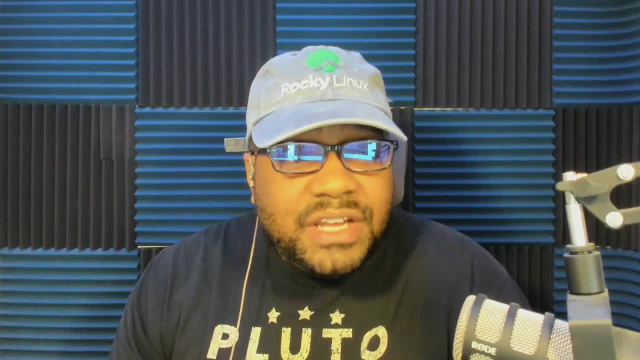 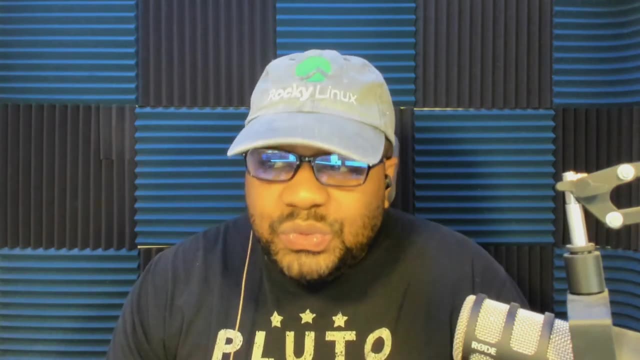 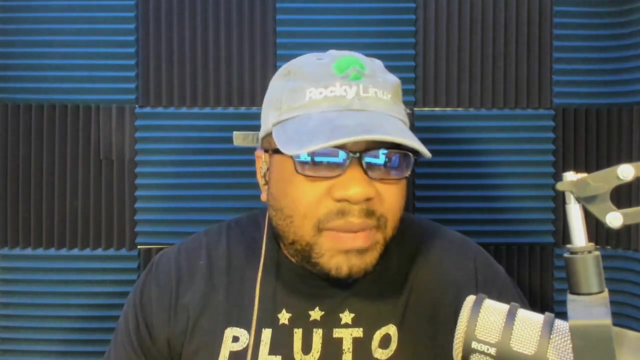 want to say this as well about Tails, even though it provides a high level of like, privacy and anonymity, but no tool or software can guarantee complete security and anonymity online. it's all about the appropriate precautions that you take, as well as following best practices while being 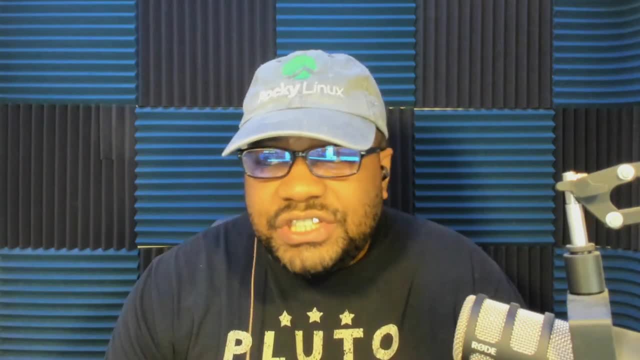 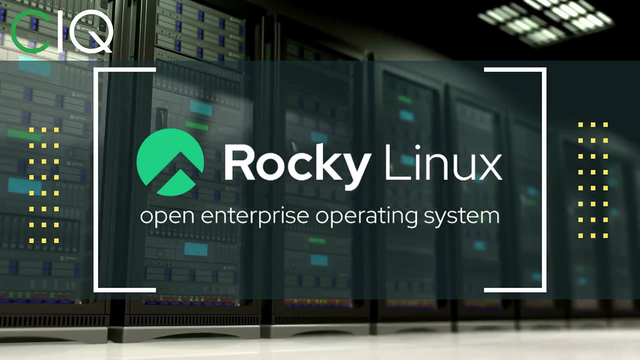 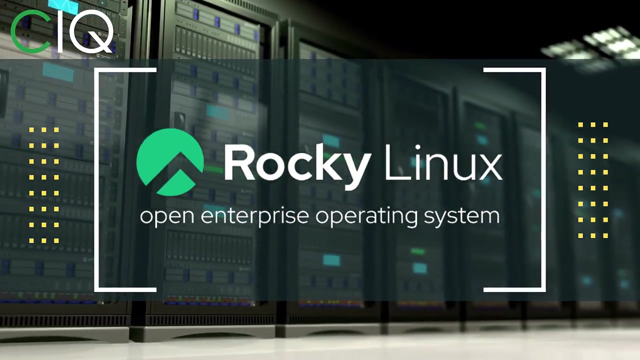 connected to the internet. so let's hop over to the website so I can show you guys everything about the Tails operating system. so let's get over there now before we move forward. I wanted to give a quick shout out to CIQ, the official partner of Rocky Linux. Rocky Linux is a Linux distribution. 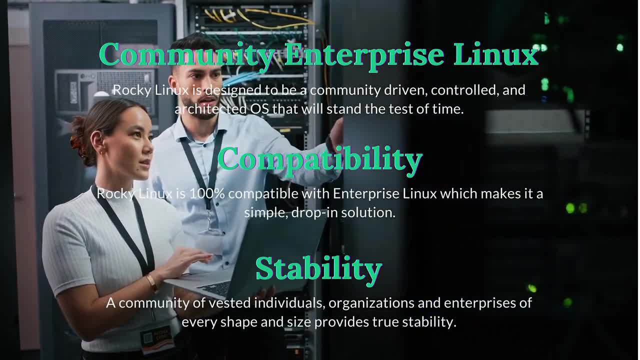 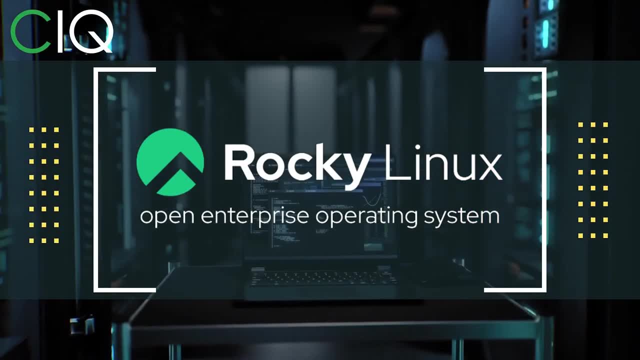 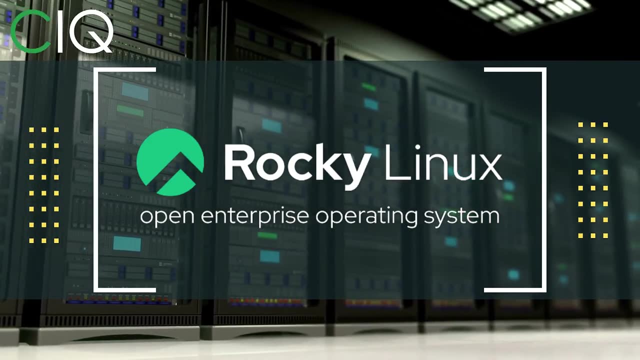 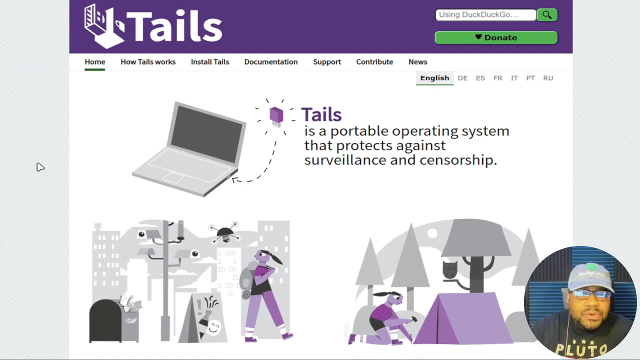 that is intended to be a downstream complete binary compatible release using the Red Hat Enterprise Linux operating system source code. the project is led by gregory kertzer, who was the founder of the senos project, so check out rocky linux at ciqco. all right, so we are at tailsboomorg. that's the link, and, of course, 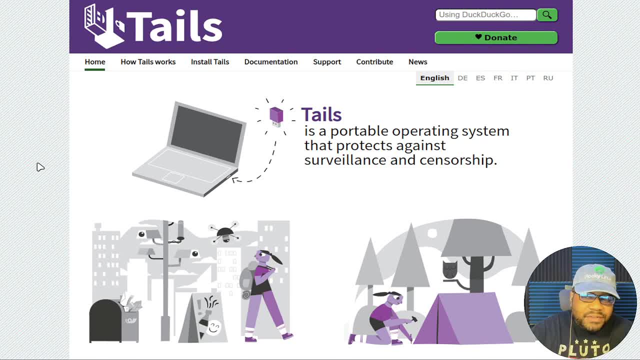 i'll always have that link down description of the video, but right off at the top it says: tails is a portable operating system that protects against surveillance and censorship. that's specifically why it was built, and you guys have heard me say this in other videos, but there are 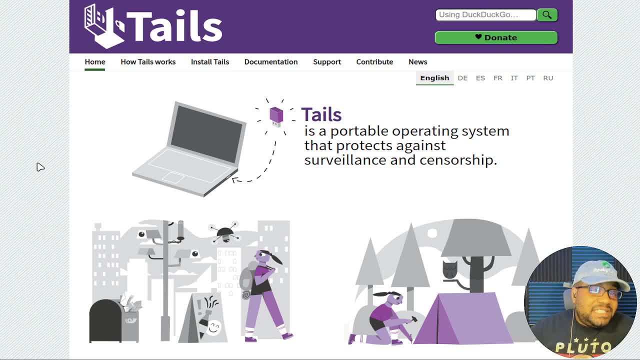 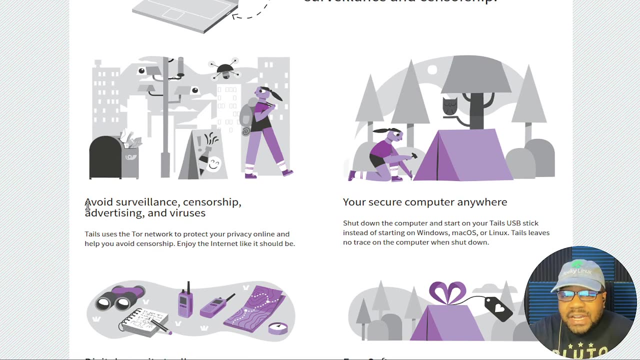 plenty of distributions out there that are built for specific purposes, and that's the specific purpose that tails was created for is to protect you. but it's all based on how you use it. but let's get a little more information. but it says: avoid surveillance, censorship, advertising and viruses. 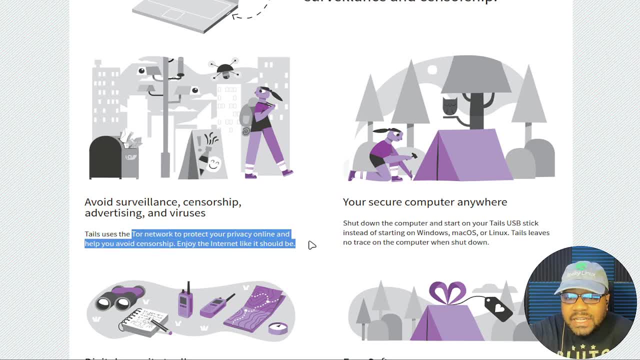 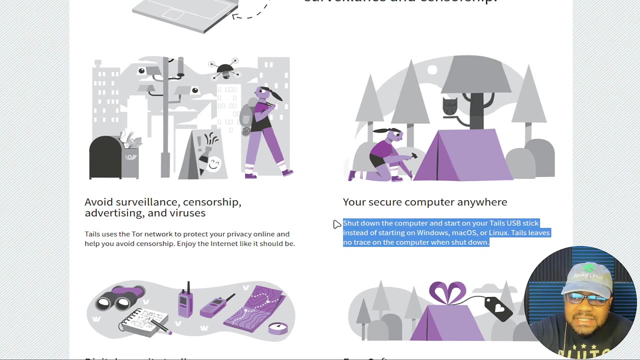 it says tails uses the toy network to protect your privacy online and help you avoid censorship. bye, enjoy the internet like it should be. you're a secure computer anywhere, so shut down the computer and start on your tails usb stick, and that's what i was going to break down to you guys. that's. 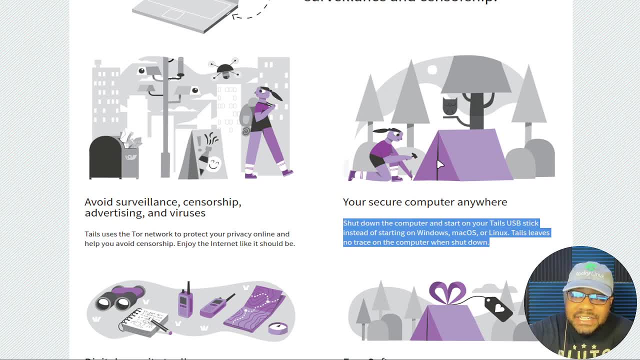 essentially how you use it. um, that's why they put a tent here or a person setting up a tent. uh, basically, you don't leave a trace. you know i'm saying: uh, by using a system you can shut down any system, plug in the usb, boot up tails, use it, use the internet. you know no one. 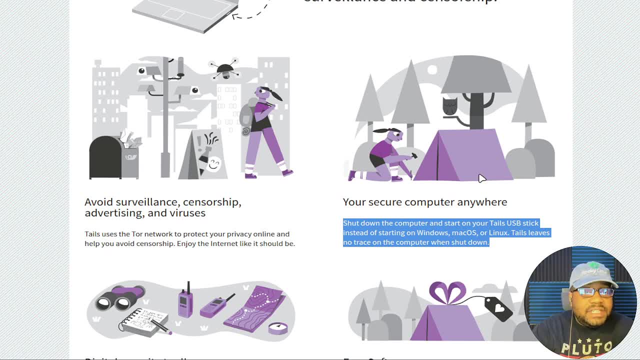 will know that you were there because you didn't access the current operating system on the horror drive for that system. but yeah, like it says, shut down the computer and store it on the tails usb stick instead of starting windows, mac os and linux. tails leaves no trace on the computer when shut down. 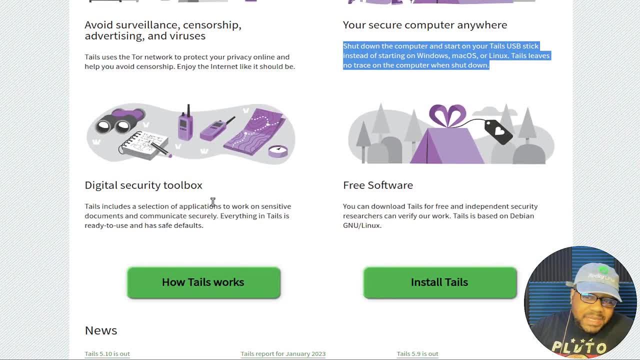 and then right here digital security toolbox and basically this talks about the tools that you have in there. so, uh, tails includes a selection of applications to work on sensitive documents and communicate securely. everything in entails is ready to use and has safe defaults, so that's one cool thing about it. 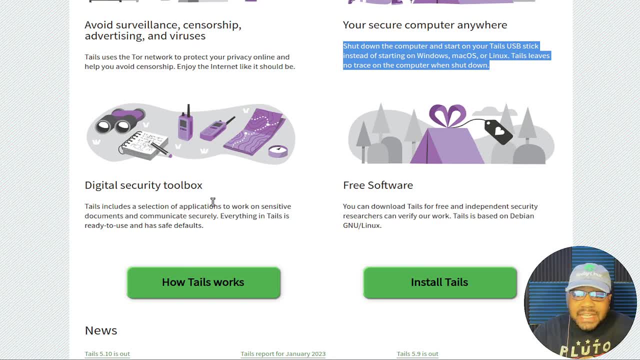 they specify that all the tools that they put into the operating system not specified, but they make sure all the tools that are included with the operating system you know have the safe settings on it to prevent you from, you know, information being leaked out in any way. it's all. 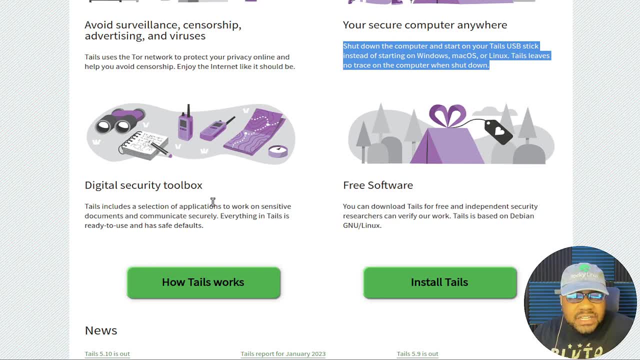 uh, going through the tour network and you really don't have to worry about it. now also, tails is a free is free software. it's free and open source. it's based on devian, and that's essentially what this is saying right here. you can download tails for free, and independent security researchers can. 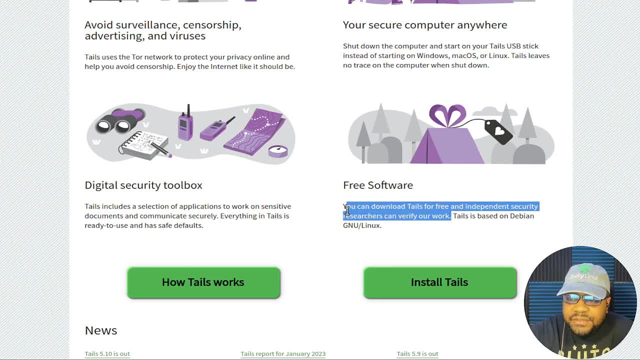 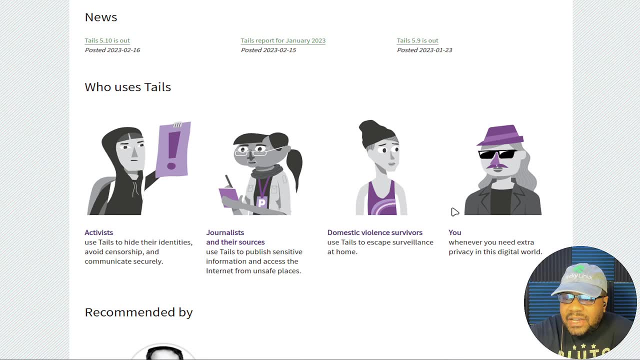 verify our work, and that's true. uh, you can verify the iso that you download. so you get to go and then down below they have a little news so you can check this out. but these are the the people that typically use it, so activists, journalists and other sources, domestic violence survivors. so 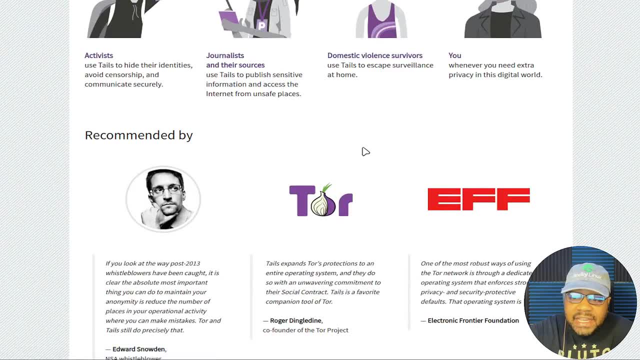 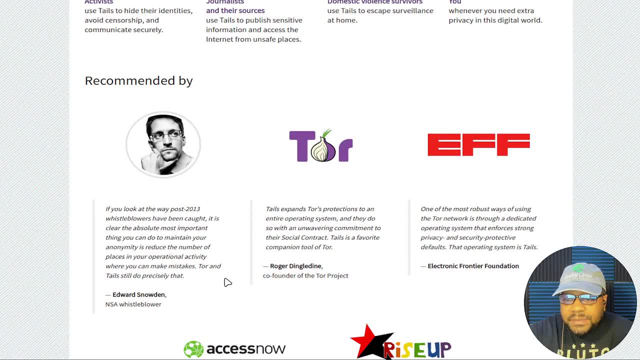 operational activity where you can make mistakes. tour entails still do precisely that, and that's from, you know, edward snowden, uh, and as well as you know, some other information or other quotes by the tour project, the founder of the tour project, as well as eff. so that's the electronics frontier. 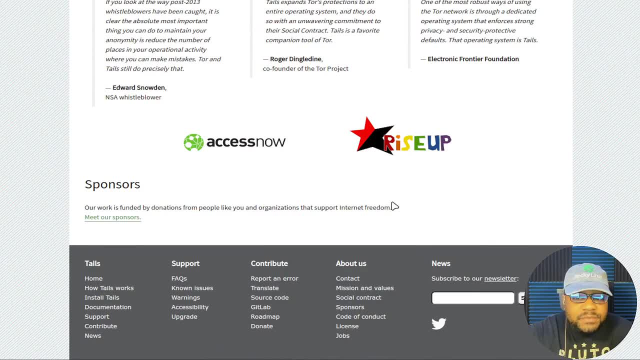 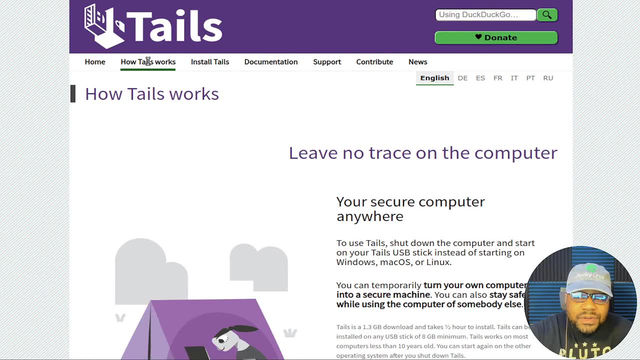 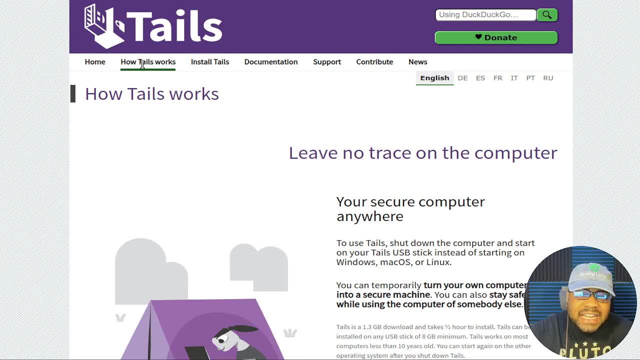 you can break. you can check this out for yourself. uh, i kind of gave you the overview of how to actually get it and use it, but we're going to get it up and going so i can show you guys everything about it. but installation, so you can go here to the install tails, uh tab. this will break down. 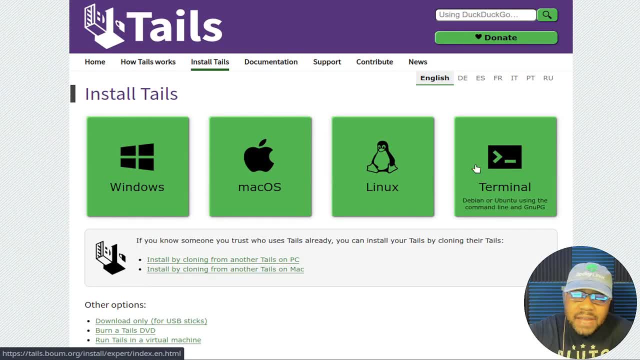 how to actually get it. just click on whichever one you're using, like whatever operating system you're using, and mainly what you want to do is clone it to a usb drive. And what I recommend is, if you want to put it on a USB drive, make sure it's a pretty decent size USB drive so you can set up persistence, because you do have an option for persistence in order to store like documents and certain things on it. 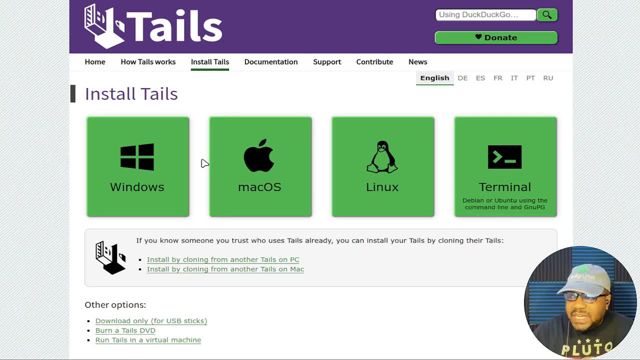 Because, like I said, it's a one time use distribution or one time use operating system. Anything you open up, run save on a system will be wiped out every time. you, you know, restore the system, So you start fresh every single time. unless you set up a persistence drive, which some people do in order to store documents, as well as other files, passwords and all that stuff, You can store that on the persistence drive. 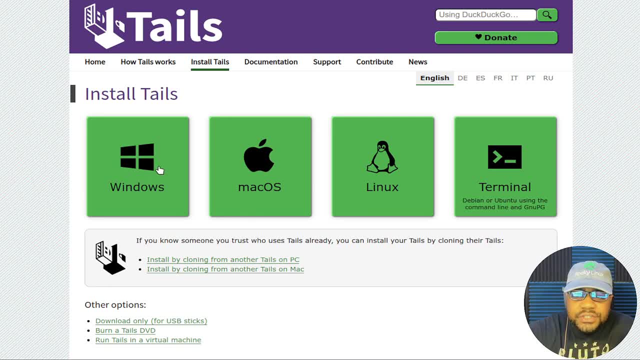 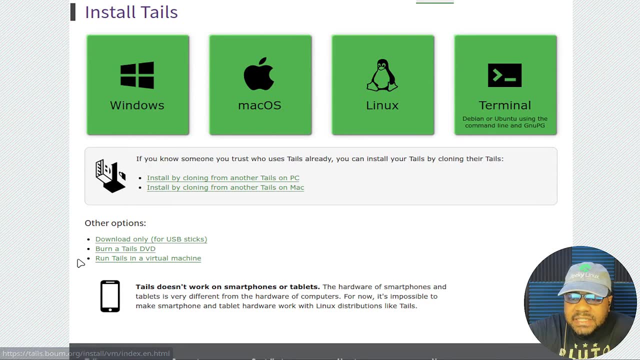 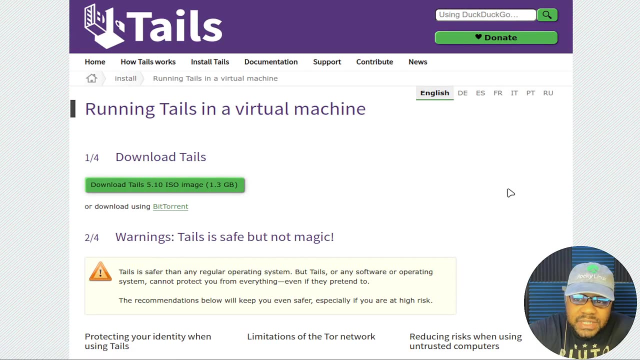 And, as you can see right now here, you can click here. This will walk you through how to install it on a USB. Now you do have other options. You could download only for USB sticks. You can also burn tails to DVD. That's another option. You could also run tails in a virtual machine, which is a good way of doing it, And that's the way I'm gonna show you guys how to do it here. 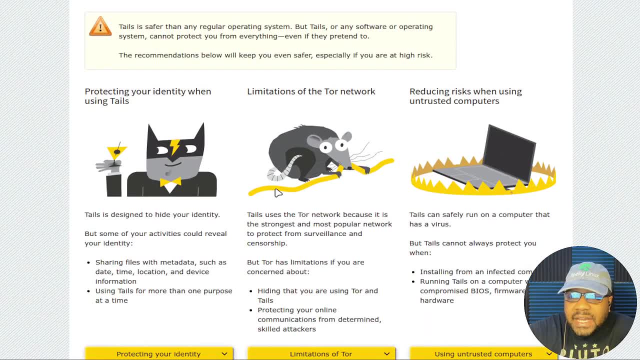 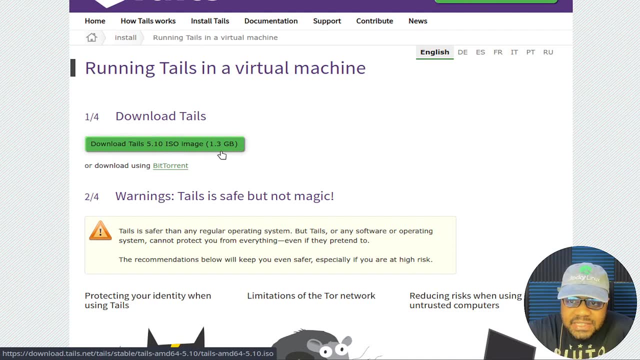 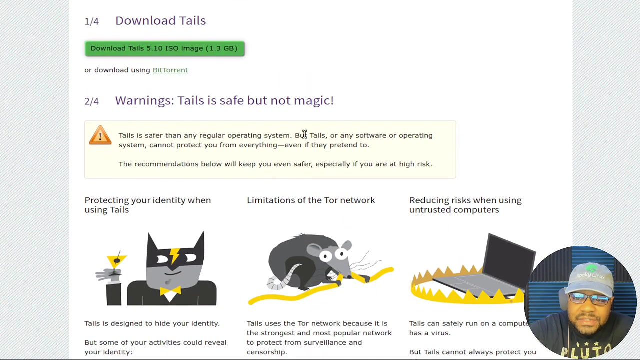 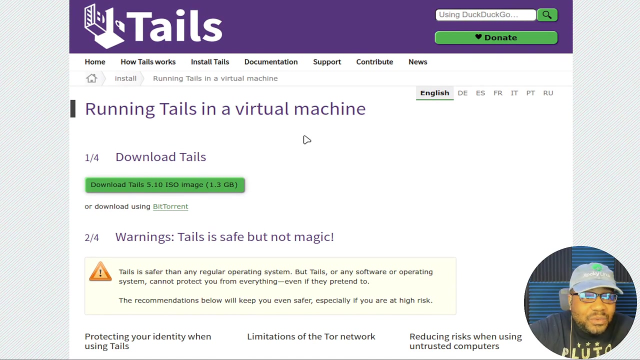 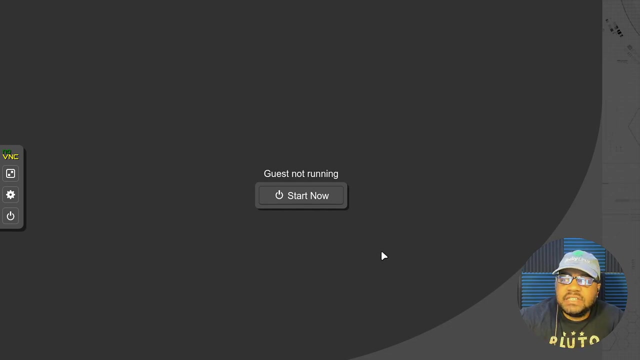 And I won't set up persistence or anything. I'll just walk you guys through how to get it installed. But you can download it right now. They're currently on version 5.10.. It's 1.3.. 3 gigabytes, So I recommend getting like a 20 gig or a 30 gig USB drive in case you want to save some files on it or whatever. But yeah, this is a super cool distro that'll help protect your identity online. Now let's hop over to my virtual machine so I can get this thing booted up and we can walk through what it actually looks like and how to use it. Okay, cool. So I created a virtual machine And just so you guys know, 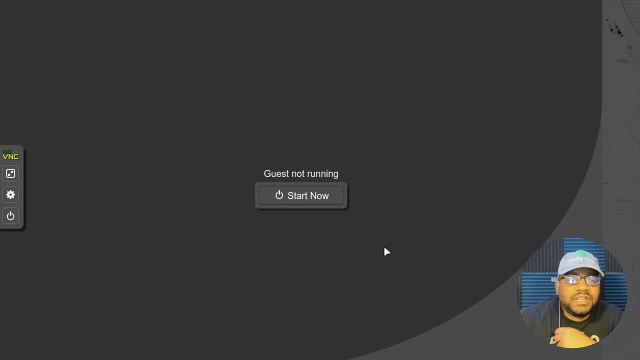 you don't really need much hardware because it's going to run everything from the CD. But I put some hardware on it anyway. I think I gave it like 32 gigabyte hard drive as well as eight gigs of RAM, So it'll run pretty good on the system. I mean similar to you plugging it in to a real system. But none of that actually matters because it's not going to write anything to the hard drive at all. It's going to run everything from the USB. So 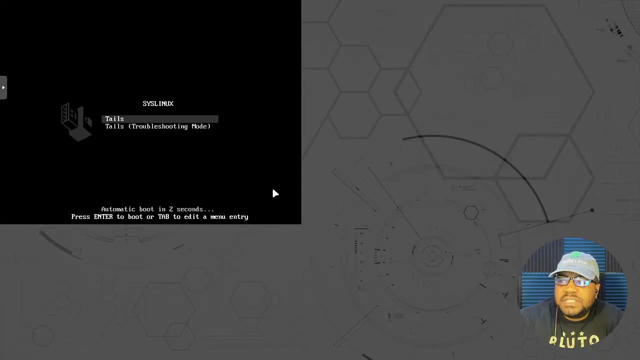 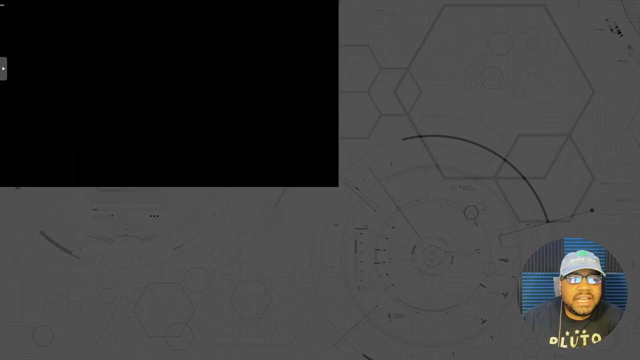 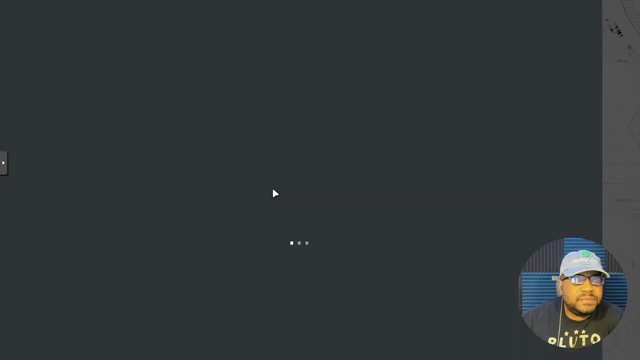 it's going on and start this distro And I wanted to show you guys the first things that will show up there. It's basically a tails and a tails troubleshooting mode. we're going to just go to the tails version. If you need to troubleshoot, that's what that's built for right there. So let's go down, press enter there. It'll automatically go to that. I just stopped it. I think it's a countdown in there, But it'll go on and boot up the operating system And, depending on the hardware, it may take some time, But most of the time on. 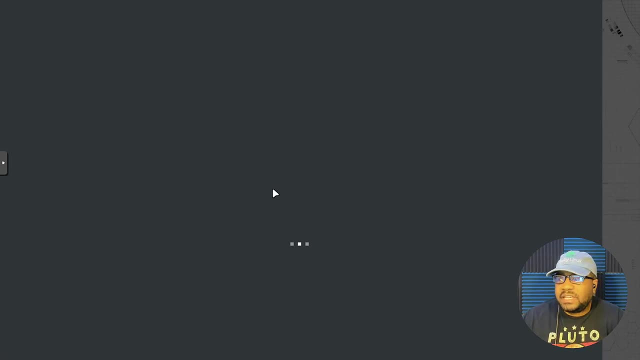 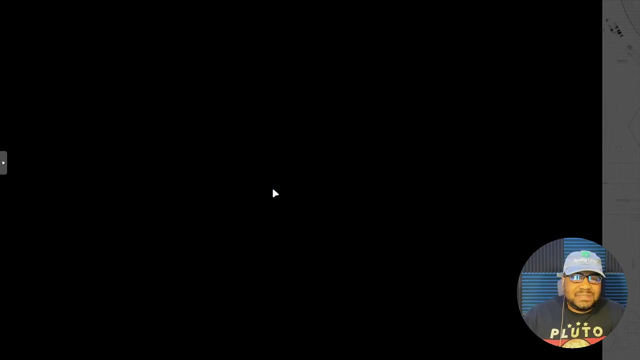 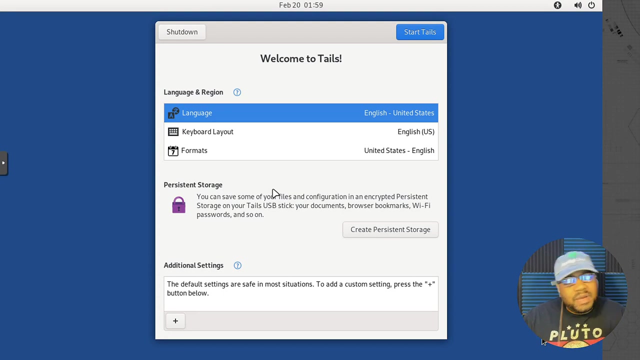 and usb drives. you know it'll boot up fairly quickly, but like on a dvd uh- which a lot of people don't have cd drives or dvd drives anymore- it may take some time because that technology is getting older now and so it's slower to boot up, but this is the first thing that will pop up and 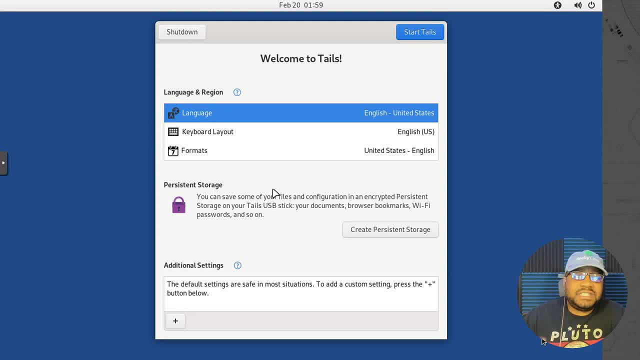 that's what i wanted to show you guys, and this will pop up every single time you boot up the operating system. just so you guys know, because, like i said, this system is fully live. you know i'm saying it's not saved in any way. you can't install it, it won't pop up with an installer. 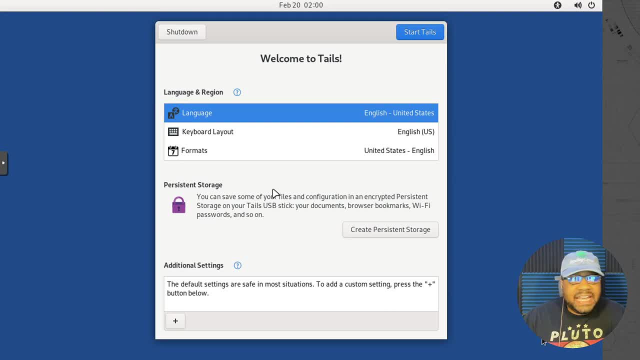 and it's made to run as if you downloaded it today. you know every single time. but just show you, guys, a few of the options here. you do have shutdown, you have start tails right here. that'll start with the settings that that are set here, and what it'll do is it'll just put the defaults. 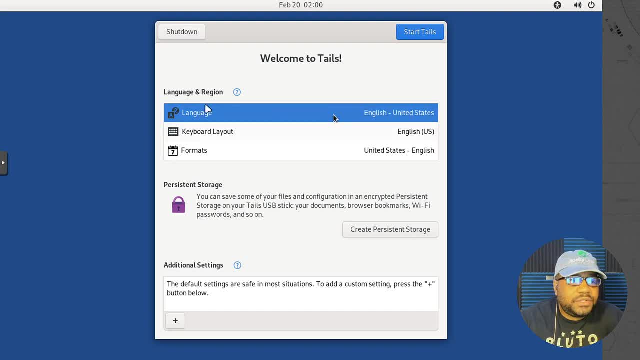 in here which is english. uh, and that's the language. so you can go in and modify this. so if you need a different language, all you have to do is click here. boom, you can find whatever language you want. add it, change it. that'll change the language of the operating system and then the 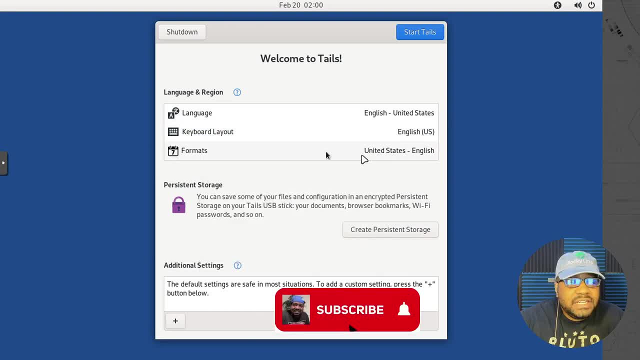 keyboard layout. you can change that as well. all you gotta do is click on it and any format. this is, you know, just your formats for everything. so we're gonna use united states english for me. so the defaults work for me, but if it doesn't work for you, you can go down and change it, depending. 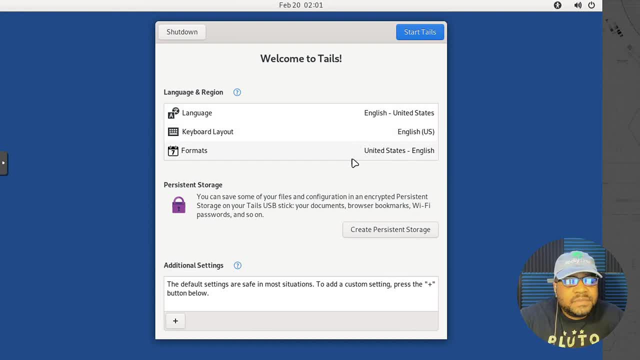 on your location, what language you speak. you know all that good stuff. now persistent storage. this is one of those options i was telling you about. uh, you can set persistent storage, and i'll just read a little bit what it says right here. it says you can save some of your files and configurations. 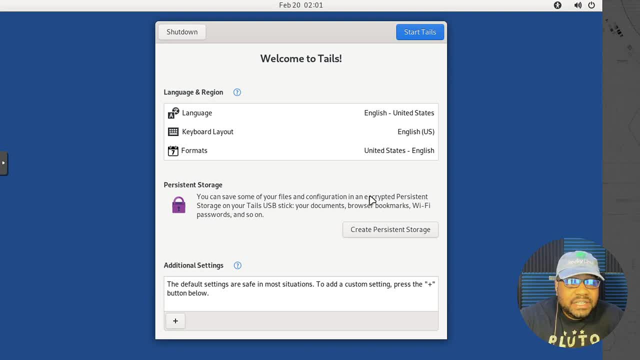 in an encrypted persistent storage, and this is the key word right here. it's encrypted, so you don't really have to worry about anybody getting access to it, because it's going to set a password and as long as you don't set up an easy password, it's something you can remember. you know you can get. 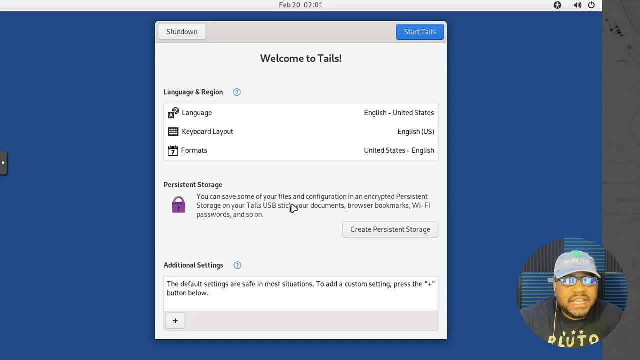 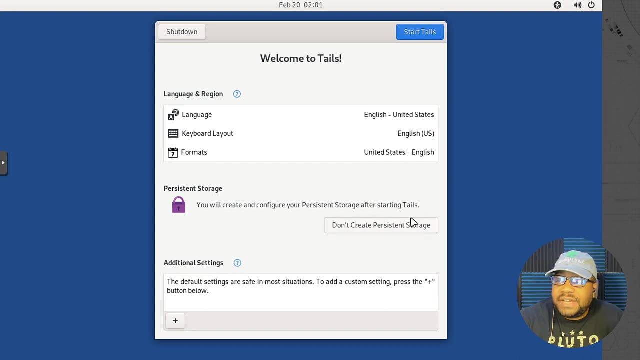 into your persistent storage one the usb drive, and it'll be stored on the usb stick when you uh create this uh. so all you have to do is hit create persistent storage and right there it'll say: you will create and configure your persistent storage after starting tail. so after it boots up the operating system, you can set up. 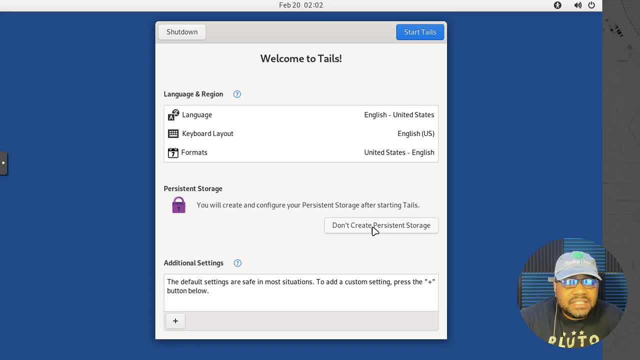 your persistent storage. uh, with a password, all that stuff, it'll be encrypted. i'm gonna just turn it off for right now, because we don't need it now. there are some additional settings- uh, you could change, and what i want to do is show you guys what it is. 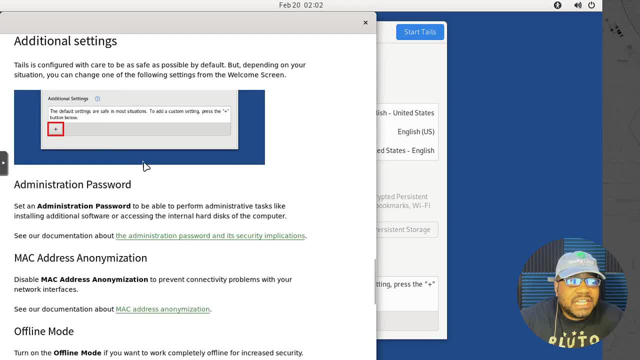 uh, by clicking here, this will open up the help so you can check out exactly what they're talking about. under the additional settings- now, uh for one- you can set up a administrative password if you want to. uh. mac address anonymization so you can disable that. uh, this will disable the mac. 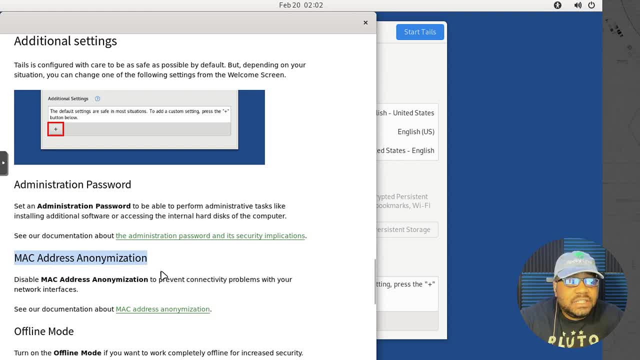 address anonymization, but by default it keeps that on. you know, i'm saying, and if you guys don't know, the mac address is basically what identifies the hardware of the system. uh, it's identification id for the network device of that computer. every network device that's produced has what they. 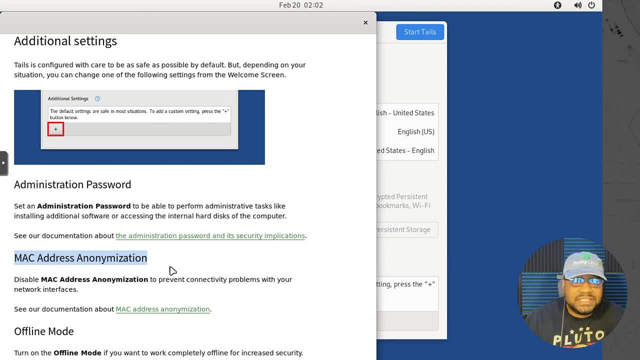 call a mac id and most of the time it's different from anyone in the world. but i'm sure some manufacturers probably have used the same ids, you know, for mac addresses, uh, but the mac address is typically different, you know, per each device on each system. as far as the 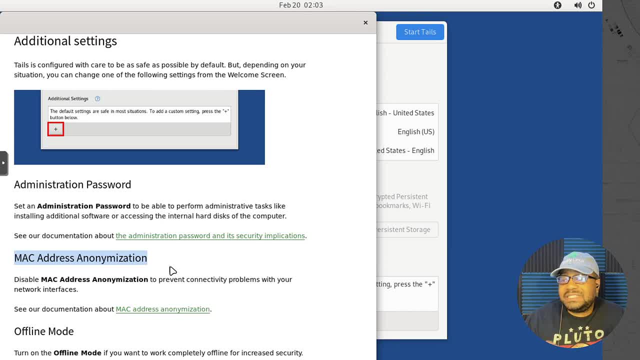 internet device that's on your system but by default. what this does is it anonymizes that mac address by changing it to something totally random so people can identify the system that you were actually using uh tails from or whatever you're doing on the system. but you do have that. 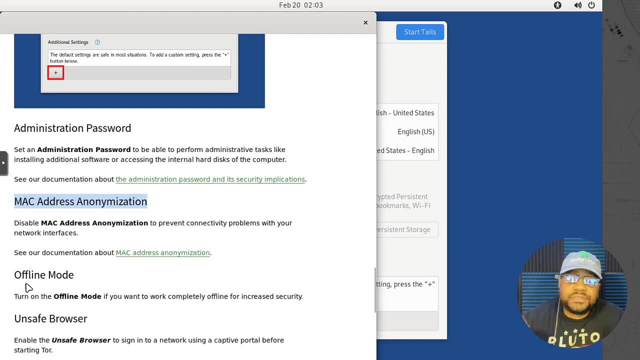 option to turn it off and then also we have an offline mode. this will allow no internet connection. this is the highest uh security you can set on the operating system. if you don't have it, any internet access, nothing you do on that system can be, you know, monitored or seen, because you're. 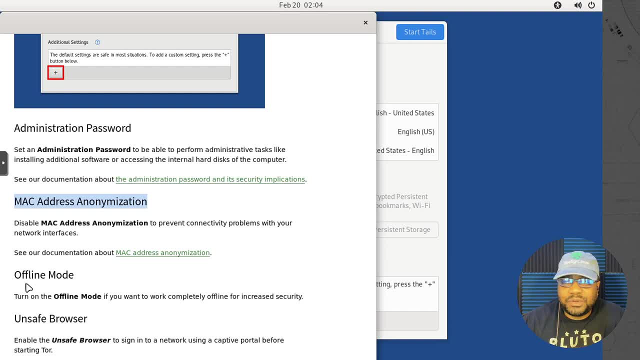 not connected to the internet at all. that's the offline mode. you can set that um and that's this. this is only for this one boot up. you know what i'm saying? i want to keep reiterating that this is just for this one boot up of the operating system. and when you go back, when you log out of it, 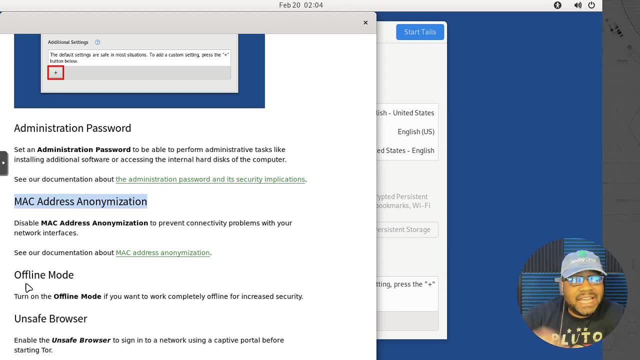 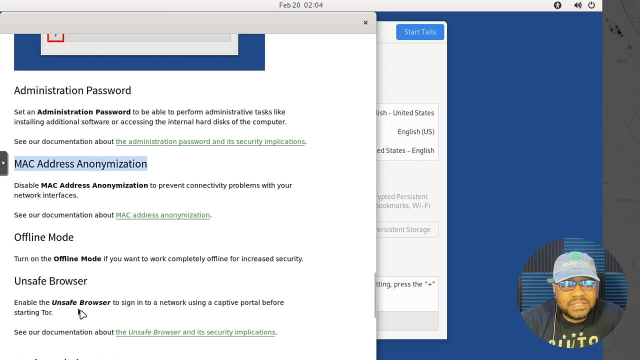 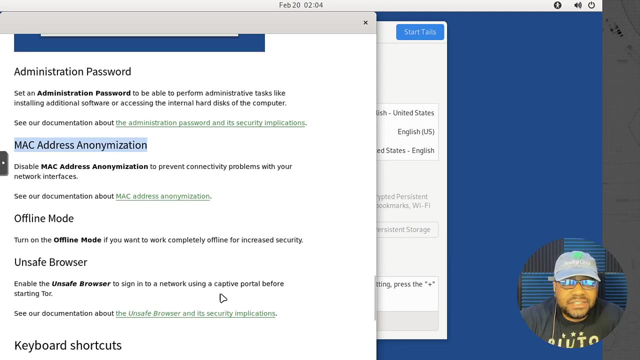 or shut it down, boot it back up. it'll ask you if you want to turn that back on or not. so it's only for that one instance. and then we have unsafe browsing. so you turn that on if you want to. that'll allow you to not use tour for everything, and so that's those options and 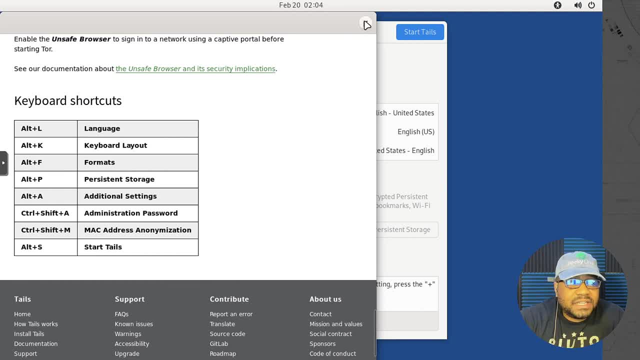 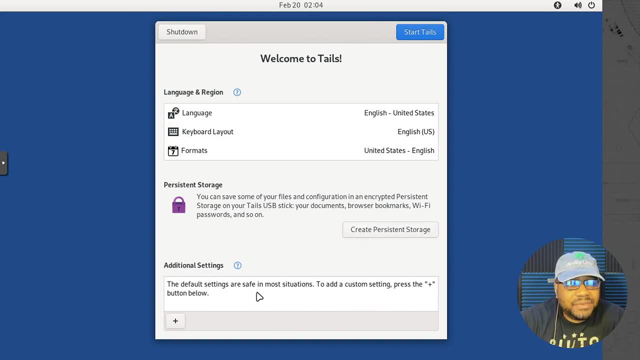 then they also have some keyboard shortcuts and all that stuff that you could modify or change, you know, for the system. now we're gonna not gonna make any settings down here in any way. no additional settings. we're not gonna set up persistent storage yet. uh, i'll probably make. 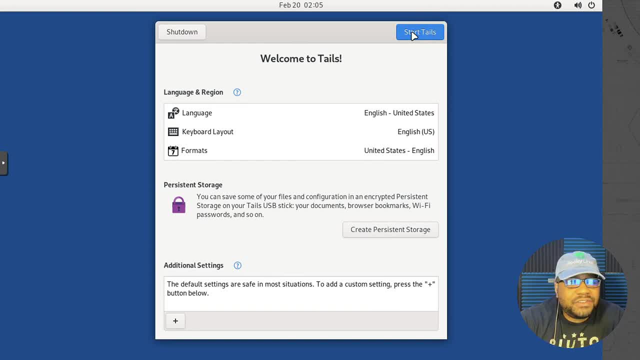 another video about that. um, that anges, and we might go back to that one more time in the future. by, uh, until they provide some Messiah. I do want to support what the mac address: um但 uh, we gonna just showing you guys persistent storage. uh, by itself, but let's go down to storytel, so you guys. 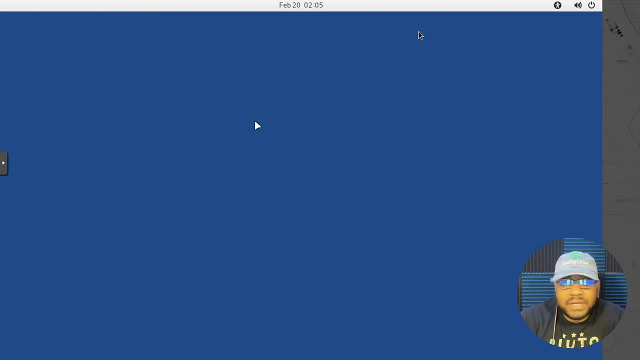 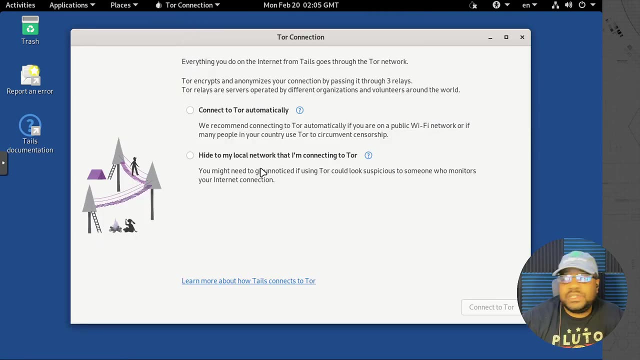 can see what it does, and now it's going to boot. it boot up with all the settings that we had, you know, set there, which we didn't make any changes. uh, and this is what it'll boot up once you, or this is how it will boot up once you- get into the system. now, what i did was i went in and 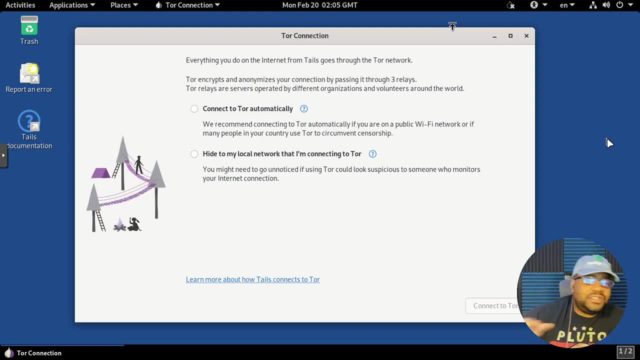 changed the display settings so it'll, you know, show right while i'm recording, but this is the first pop-up that'll pop up. it's basically telling you how you want to connect to the internet. uh, everything you do on the internet from tails goes through the tour network, and so these are. 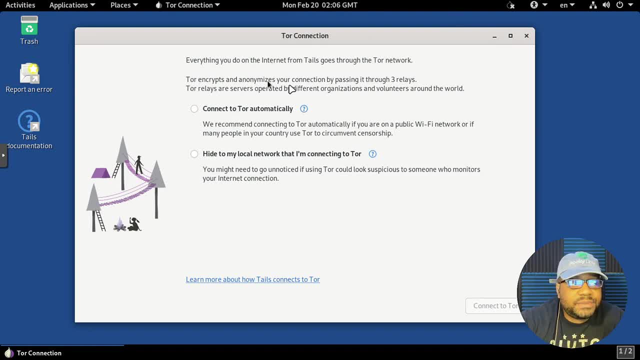 just some of the options that you have. uh tour encrypts and anonymizes your connection by bypassing through three relays. tour relays or servers operated by different organizations and volunteers around the world, and you can actually become one of these volunteers by setting up a node. 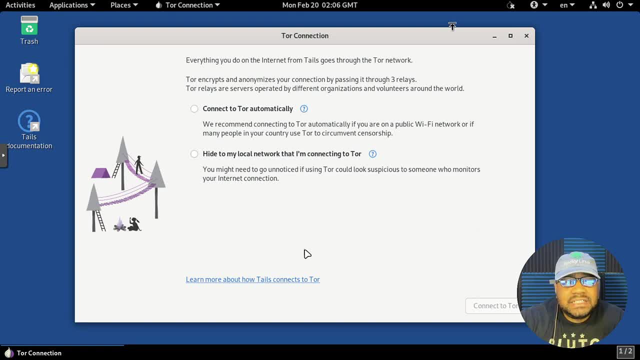 and these options are mainly you to help people with, uh, censorship. uh, in a lot of places they monitor for tour traffic and they don't want people to use tour. you know what i'm saying? well, it's a way to get around it by setting yourself up as a relay and you'll be the first relay in the connection to tour, and so this allows. 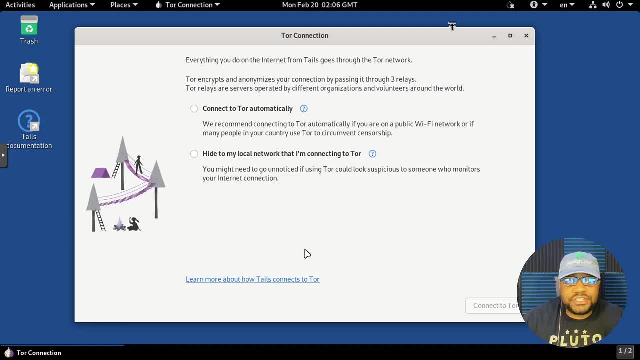 you to get on tour around that censorship that may be set up and people won't actually know that you're using tour, and that's what these two options are for right here. so right here it basically says: connect to tour automatically. so that's something we want to do, but you can also set up a tour bridge. 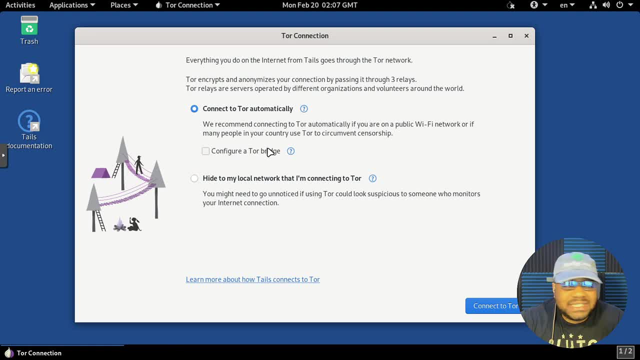 and that's what i mean by relay. you'll see, you'll be a bridge. basically that's the correct term, uh, and i'll click on that so you can see. it says tour bridges or secret tour relays. uh, use a bridge as the first tour relay if connection to tour or block. so that's the whole purpose of the tour relay. 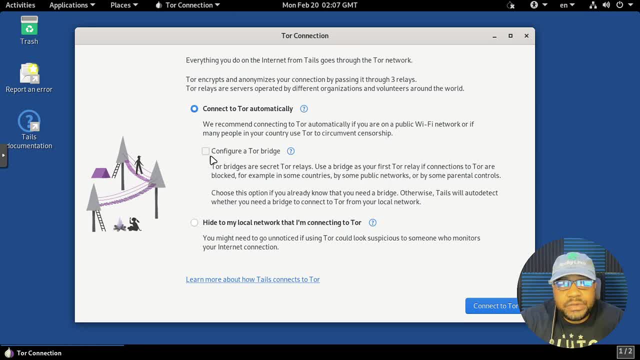 you know this option right here. you can set it up as a tour bridge or tour relay and if i click here, that'll set up that that uh relay for you. uh, now, right here down here it says: hide my local network, that i'm connected to tour. which is kind of redundant, because if i click here, 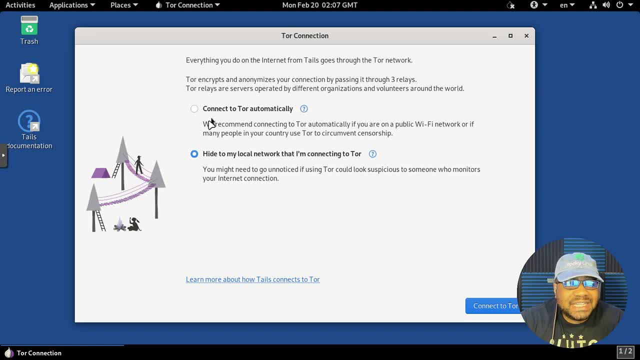 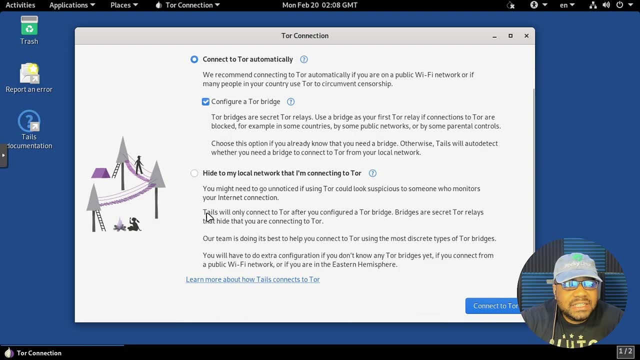 uh, that'll go away. this is basically gonna do this exact same thing as almost selecting this and this. uh, and let's click right here just so you guys can see. but tails will only connect to tour after you configure a tour bridge. you know, if you select down here, so that'll block the internet. uh. 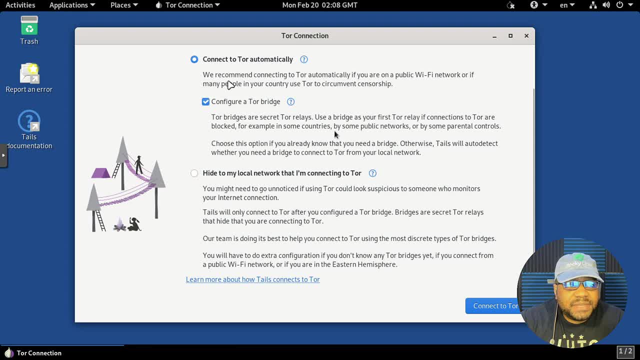 unless you have a bridge set up, and this just gives you the option up here to you know, set up connecting to tour automatically and configuring a tour bridge. but you can still connect, you know, to tour without a bridge. but this will specify if you only want to connect a tour or if you only 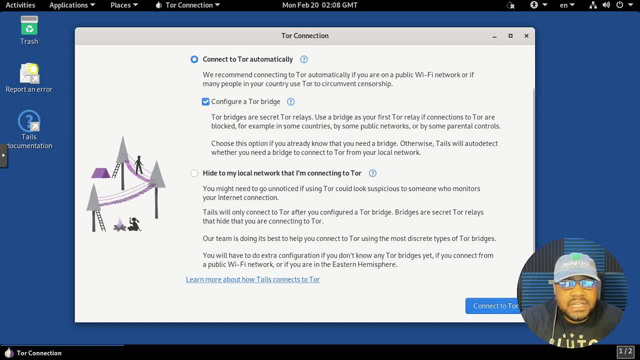 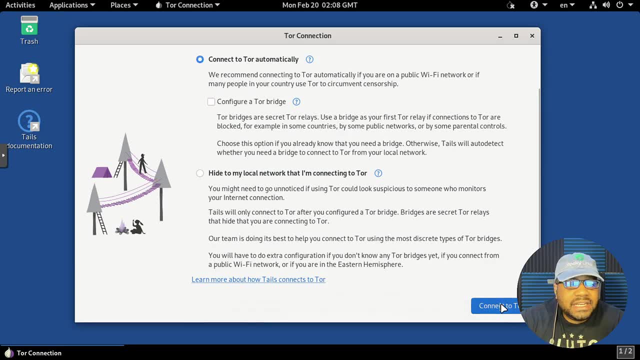 can connect to the internet through tour or not so, and so i'm gonna unselect the configurator bridge because we don't need it. i'm gonna just roll with connecting the tour automatically and hit connect the tour, and this will connect all your network connections. that's the easiest way to set it up. 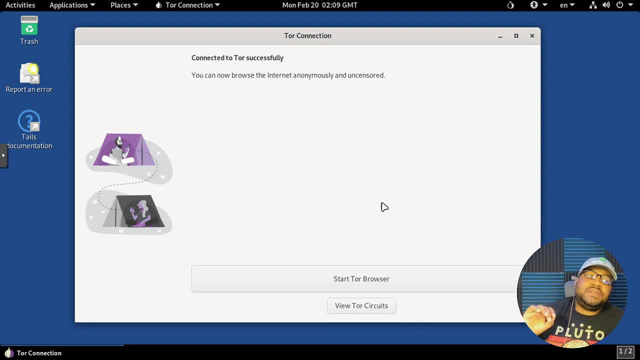 connect all your settings through tour. and one other thing about the bridge that i didn't explain, and i explained it in one of my tour videos: uh, in order to set up a, if you set up a tour bridge or a tour, or if you become a tour relay, then just know that connections will be coming through your. 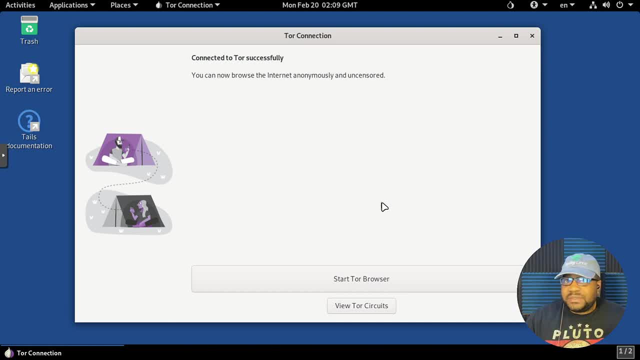 system over the tour network, because your system will be looked at as another node that people can jump to through their three layers of protection or three layers of encryption. uh, so if someone, let's say someone in greece, they are connecting to tour and they and it automatically, like it looks. 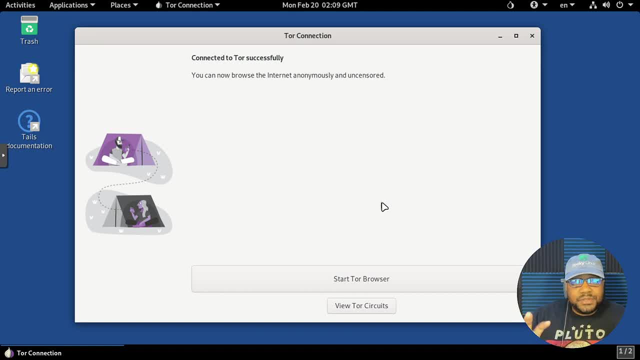 my computer. it'll it'll find my computer as a relay and it'll route that person's in in greece traffic through my connection as well. so you have connections coming in and out from different people, uh, and you know your connections are going out as well to other people within the 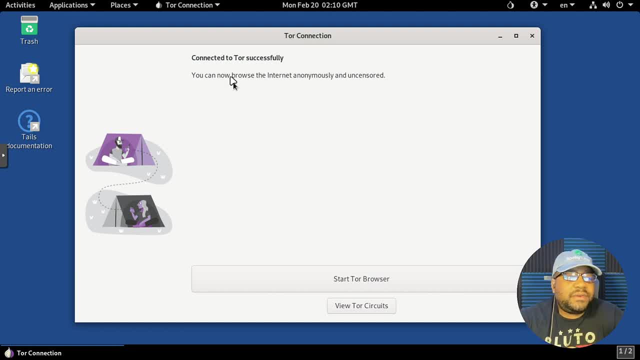 network. i just kind of wanted to explain that for you guys. now right here, connect connected to tour successfully. now you can start start the tour browser. most people that when they connect tails or start tails up, most of the time they're going to get on the internet so they can browse. 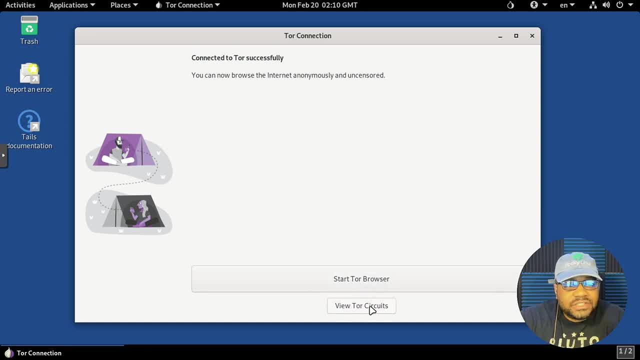 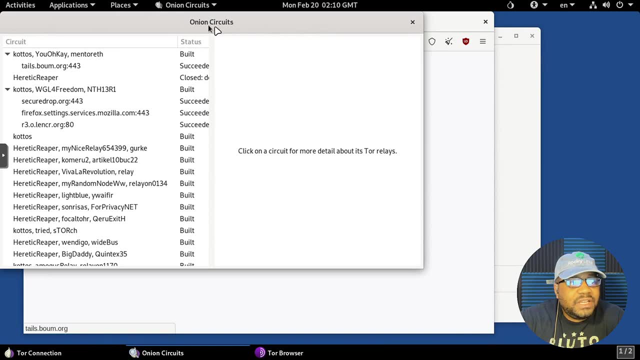 anonymously. so you can start tour browser from here. you can also check out your view tour circuits, which that'll show you guys, uh, your connections right there, so your onion circuit right here. so i don't have no problem showing you guys this, because it doesn't have my- like, my- ip address. 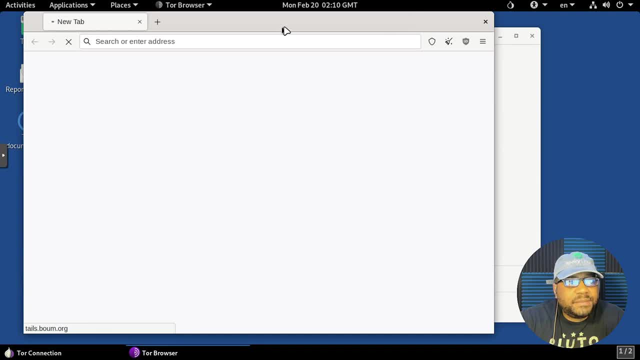 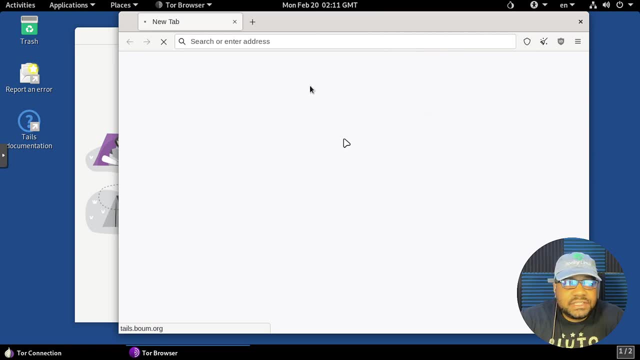 in any way, but that'll break everything up. so i'm going to show you guys how to do that. so everything out for you right there. but we are now connected to the north tour network and it'll open up the tour browser with all the security features that you want on here. now the tour. 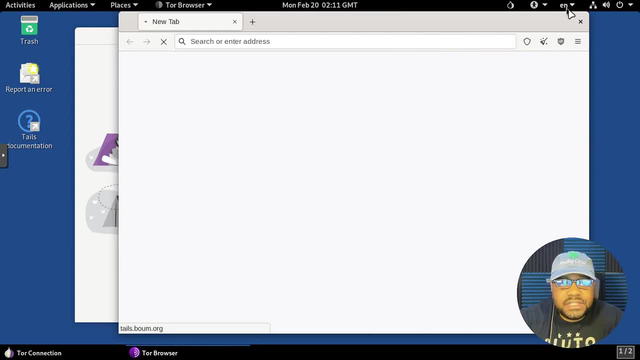 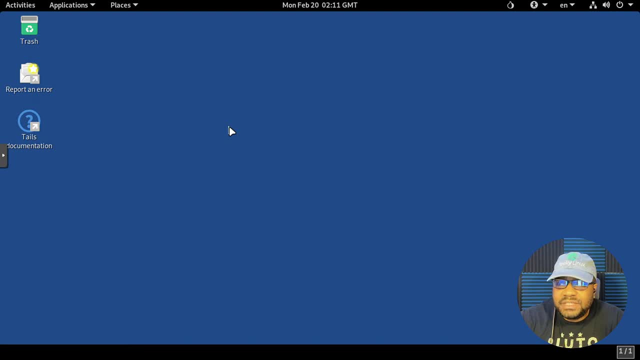 network is super slow so i'm not gonna uh wait for this to load. i just wanted to show you guys this, but that'll connect you to the tour. you can close this after that, but that'll show up every single time you log into it and just so you guys know this will let you know if you're connected. 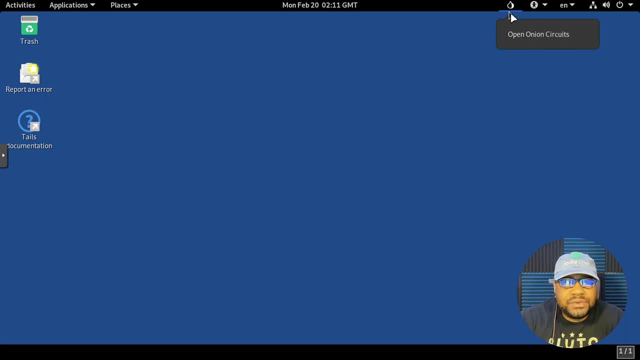 to tour. so this is your circuit it'll. it'll show you know the full onion. it won't have the x over it. so right now all your connections through this system will go through tour. now let's just break down a few of the applications that are installed on here. like i said, it has pretty much everything you need to use for an. 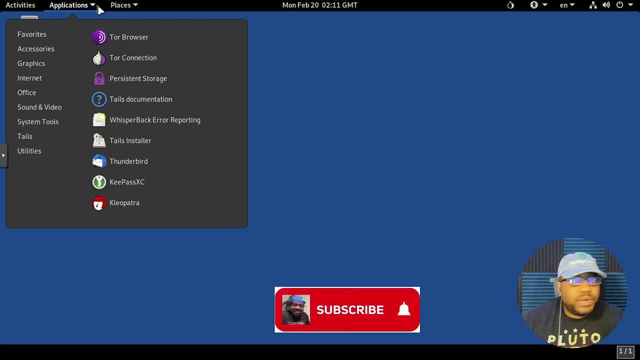 operating system and it's set to where it's as anonymous as possible. so just show you, guys, the things under favorites. this is the favorite. so you got your tour browser tour connections. you can set up persistent storage. like i said, you can set up your persistent storage after the fact. 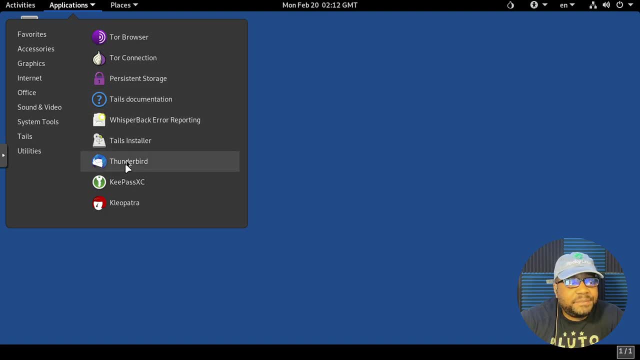 you don't have to do it. you know, in the beginning you can set it up here. uh, there's the documentation. you got your whisper back arrow reporting, so if you want to check that out, uh, tails installer so you can create another installer. um, you know, instead of downloading it from the website, you 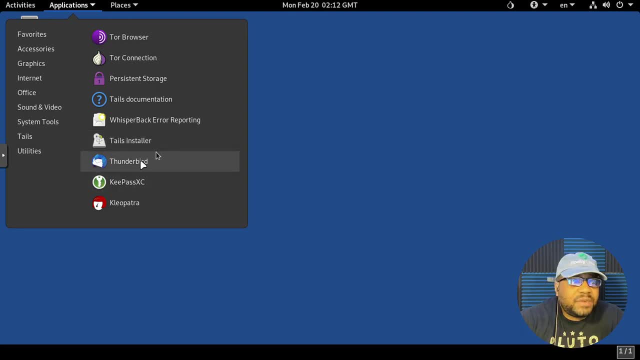 can create another one. you know, from this system, right here now you have a thunderbird, uh key pass cleopatra, so that's on there. that's the favorites. but you have, you know, normal uh file, uh, normal accessories that will pop up on any system. so you got your file explorer and, like i said, none of this. 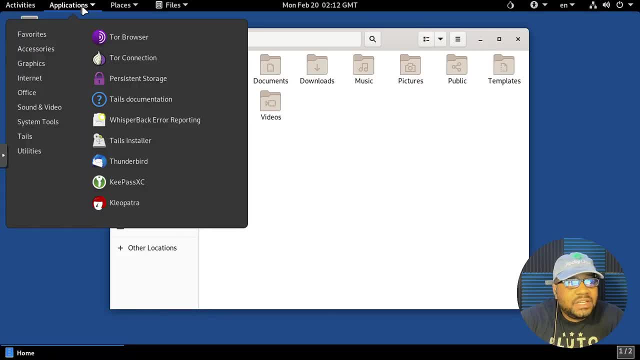 stuff is saved. so, unless you have a persistent drive, so uh, it's nothing you can do about it. uh, it'll wipe it after the fact, which is a good thing. but you can set up that persistent storage. now you got gtk hash, uh, key pass cleopatra. that shows that some of that's under the favorites. but 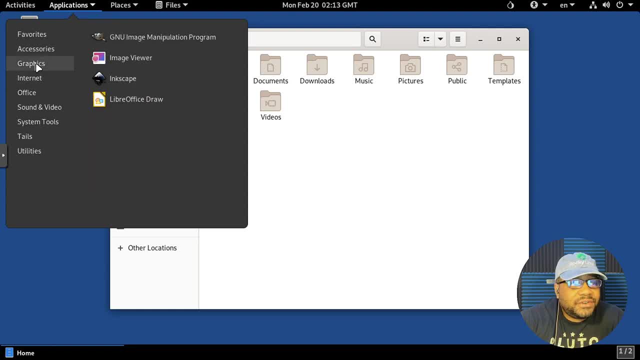 you got a data cleaner, text editor, vim, that's the one here- graphics. so you got uh gimp, which is my favorite. you know uh media editor or picture editor. you got image viewer, inkscape, uh libre office: draw um under internet. you got uh electron bitcoin, bitcoin wallet. you have onion circus. 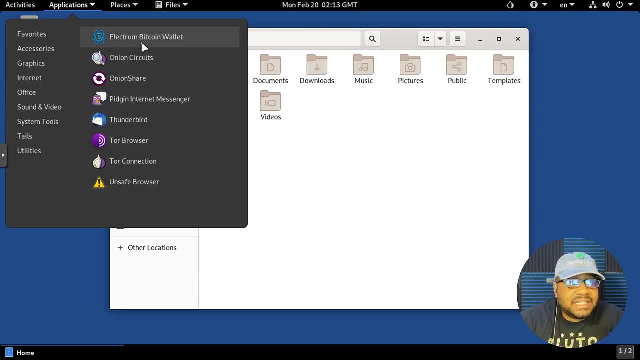 onion share, uh, and none of this stuff will be saved. like i said, anything you use on here it's not gonna be saved, so you will have to log into everything, like if you want to set up your pigeon internet, uh, messenger, you know, or something like that. it's not going to save any of it's like. 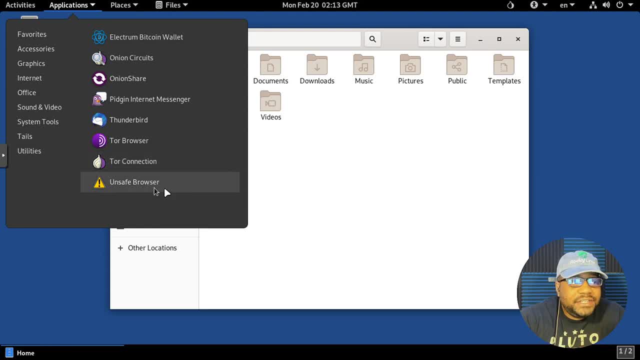 one time you so thunderbird to a browser, toy connection, and then you do have some unsafe browsers. so, uh, that's there as well. now you have some office, uh, doc, office applications as well, like libra writer, draw, calc office. you know, uh, sound, you got audacity brasio to burn this. 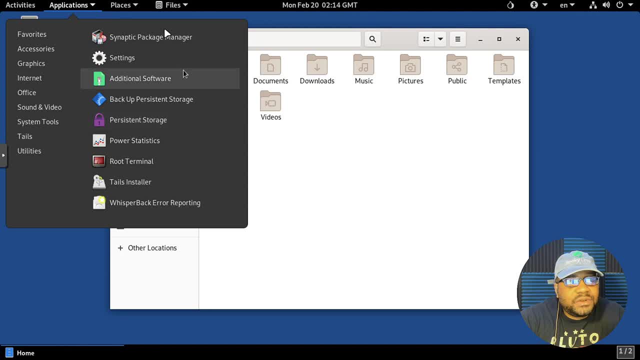 uh, sound juicer, uh, system tools. so you got your synaptic package manager on here and, like i said, if you use debian, then this is very simple to use. it just doesn't save anything and then we can go under tails. now this is where you can get your documentation. you can add additional software. 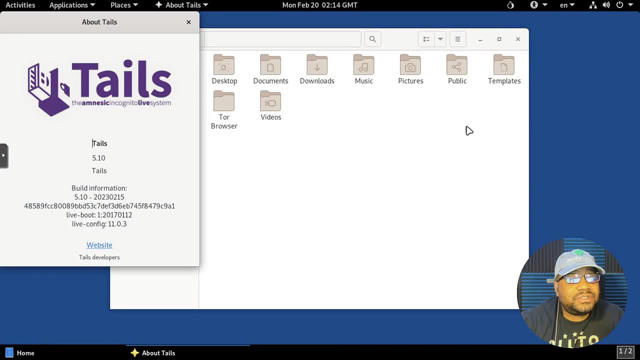 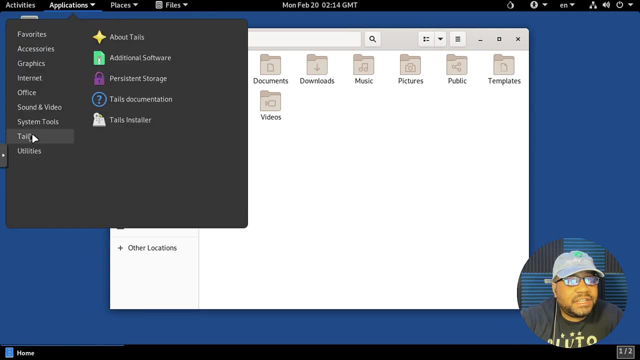 the documentation about tails. let's click on about tails. right fast, we're using 5.10 so just wanted to show you guys that. but let's go back under here. uh, but you got your tails installer. so if you need to install it to another usb you get to go. and then your utilities. so you got a terminal, you got a system monitor. 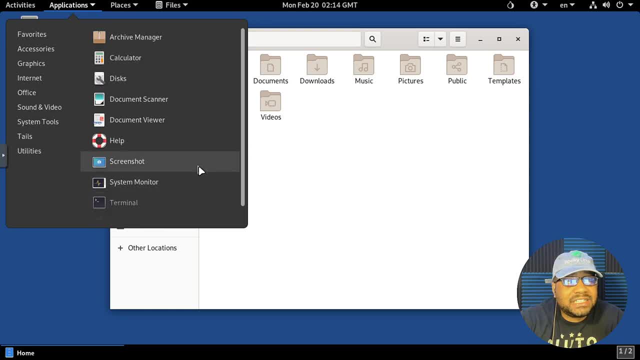 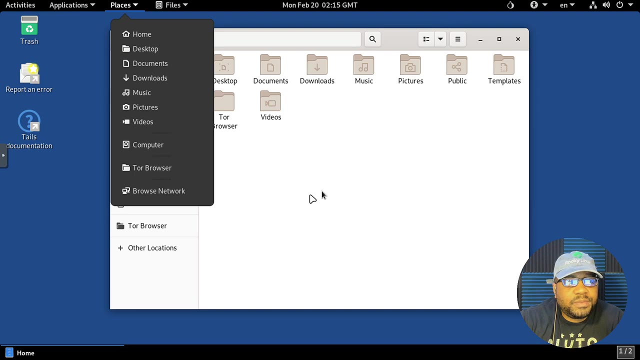 uh, crypto volumes, if you want to unlock them, and that's dealing with the persistent drives. uh, archive manager, this usage. you know all the good stuff, utilities that you want to see now under places. i didn't want to show places because it's basically this that i already had it up open. 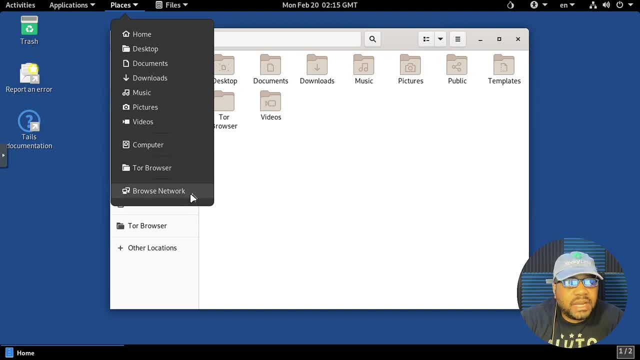 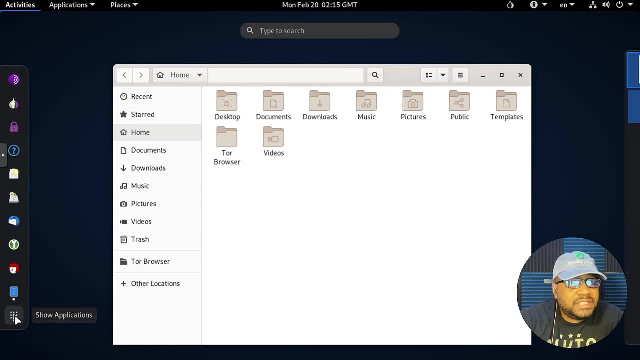 for essentially, um, and you can also browse the network. if you have something on your network- share drives, all that stuff- you can connect to them if you want to. now, under activities, this will bring up the start menu. this will show you basically all the applications that we just looked. 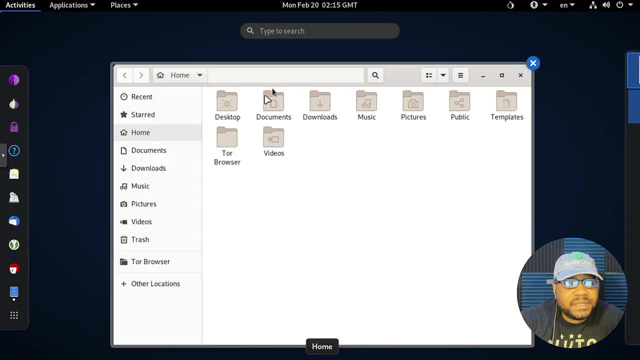 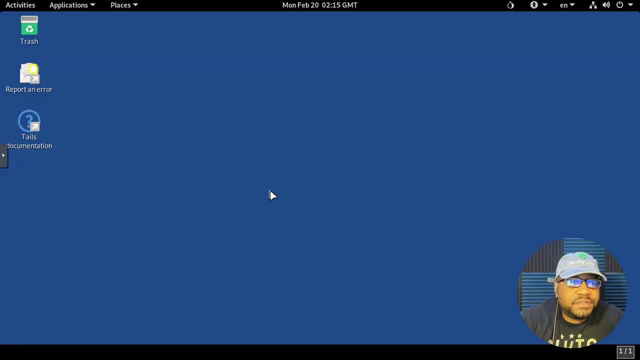 at like, like if you're using any other version of debian. uh, you got multiple desktops. if you need it, as well as the application, the different applications that are open, they'll pop up here. so if you know how to use this desktop environment, it's pretty much the same. and right here on the 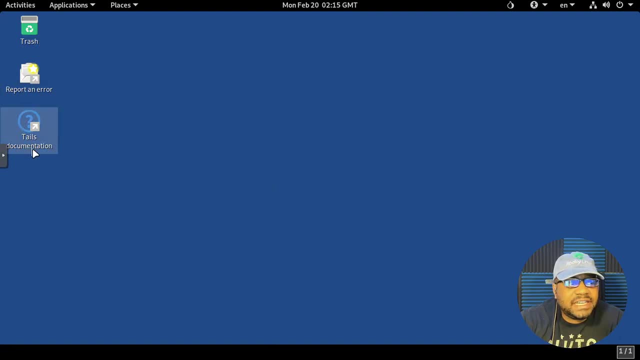 you know it'll show you the documentation again. that'll link to it. uh, report an error if you need to, as well as your trash can now just show you guys something under here. so if we go back under applications and go to system tools, i kind of wanted to show you guys these settings so we could 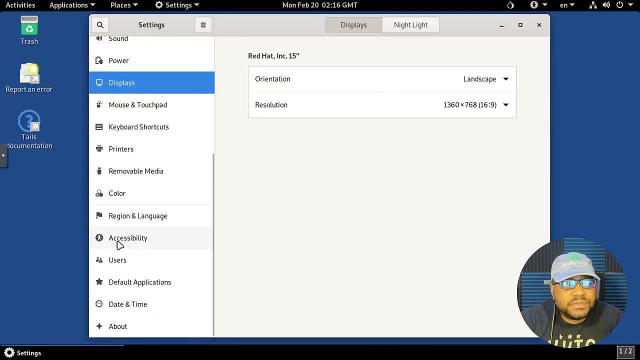 bring that up. but, bam, as you can see, super simple to use. uh, i went in and changed my resolution so you guys can see this better, but your normal system settings. but, like i said, it's not going to save you a lot of time, so i'm just going to go ahead and change it every time you boot up. so, um you. 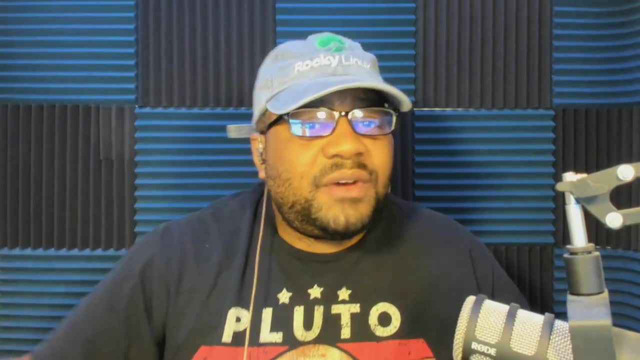 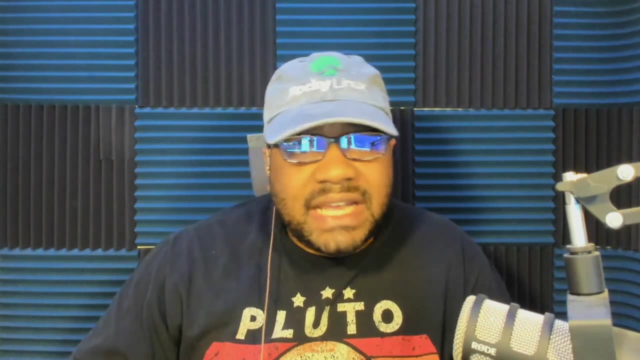 don't really have to worry about messing up anything, but that's pretty much it, so i hope you guys enjoy the video. tails is a interesting linux distribution. i definitely want you guys to check it out, especially if you want to stay anonymous online. you can use tails, you know, as an alternative. 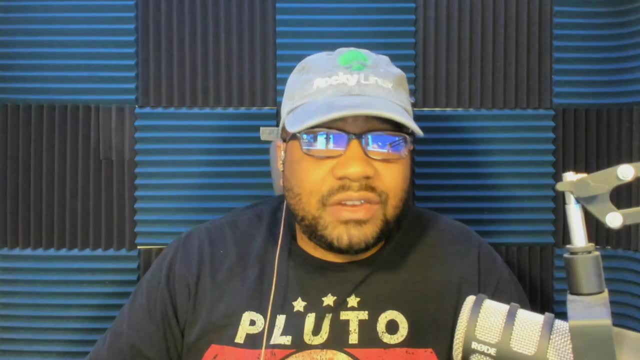 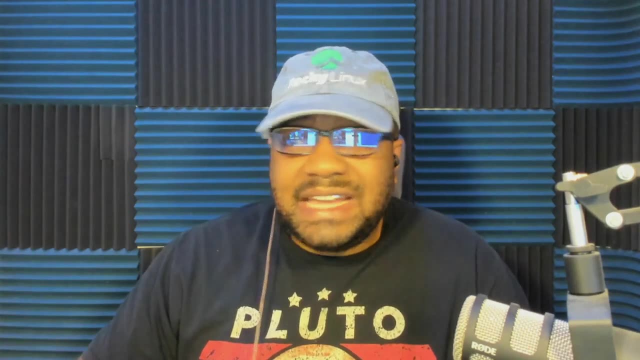 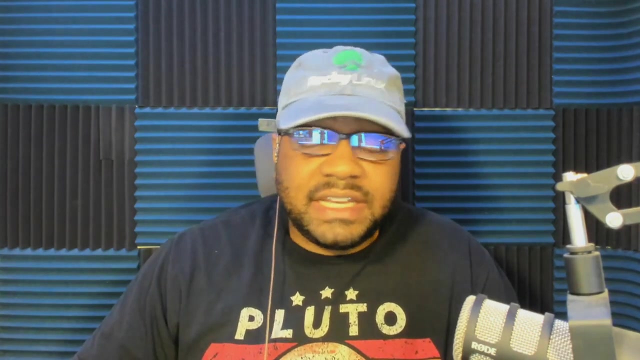 to help you, uh, stay somewhat anonymous and private online using this linux operating system, but at the end of the day, uh, this is not 100 way of staying anonymous. you have to change the way you use the internet really and to change your mindset on how you use things like logging into. 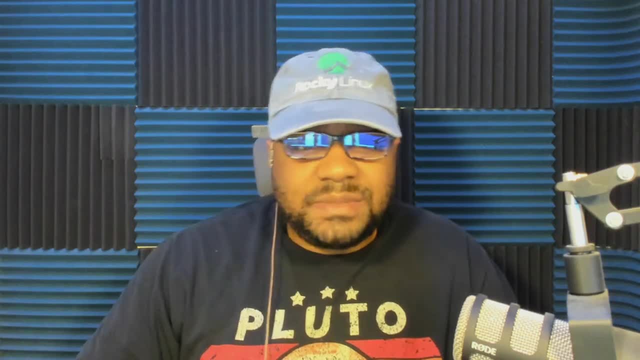 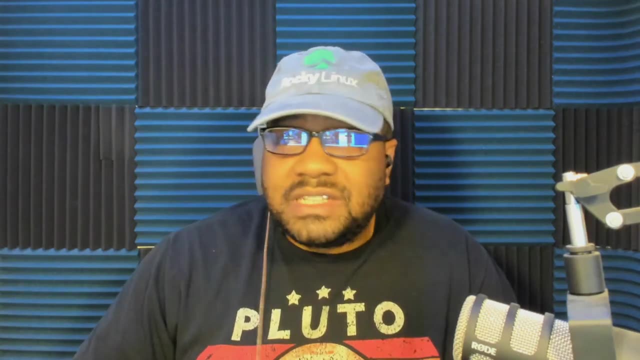 social media and all that stuff. so, like i said, it's not a hundred percent. if you get on tails, log into your facebook or something like that, then obviously someone is going to know exactly who you are because you're logging in to your facebook account. uh, these organizations, they 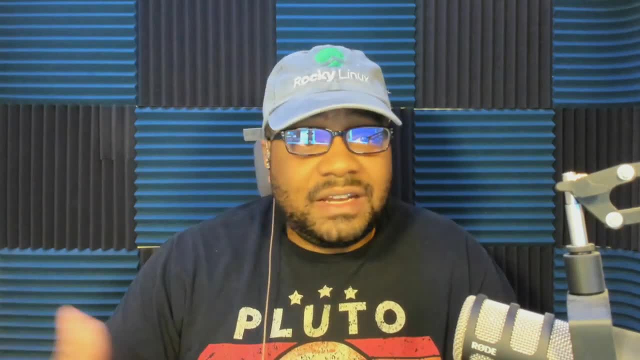 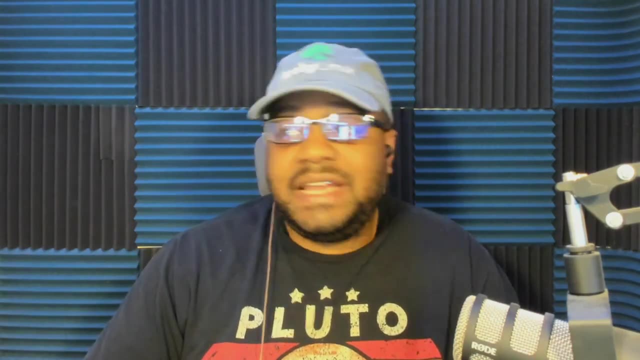 think you do so. if they see that you're logging in from this system- uh of tails- then obviously someone is going to have a record of you actually using this operating system and the location ip addresses, because you know when you log into these social media accounts they want you to.